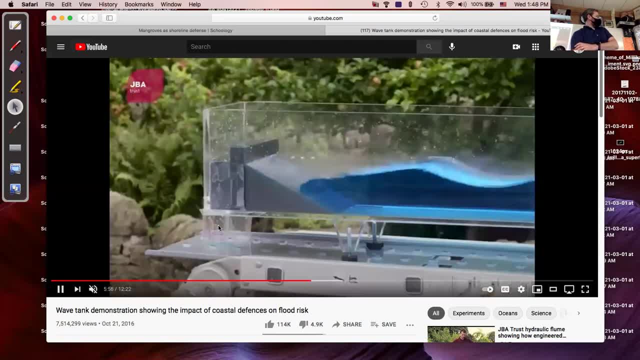 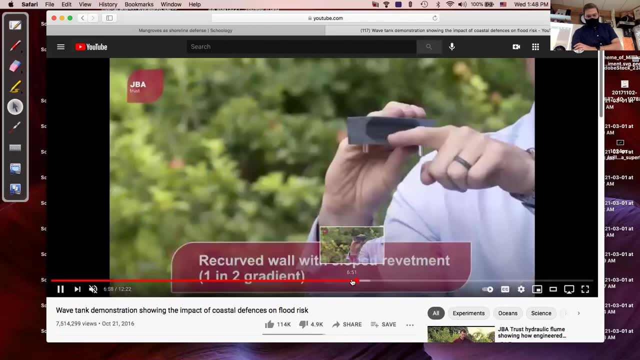 want to watch the whole thing. it actually collects some volume of liquid in a little beaker here, so you can quantify the amount of water that comes over in each of the different cases. another thing you can do is have a- uh, a recurve wall or a return wall, and these are used in some areas too, where 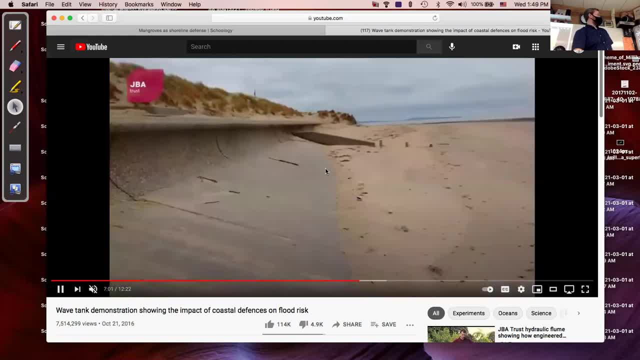 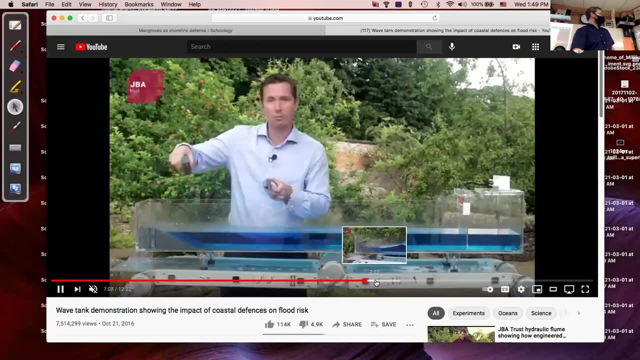 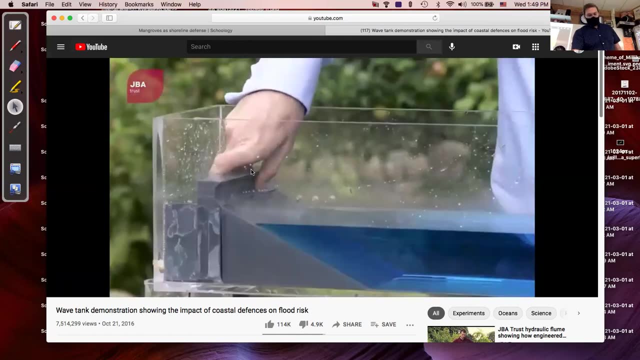 you put: uh, this curve shape. so when the waves rush up against here, they hit the curve and they splash out toward the sea and that's very effective. but it's a lot more expensive to build and they're highly susceptible to erosion, and if the water overruns it then it doesn't really help a whole lot. 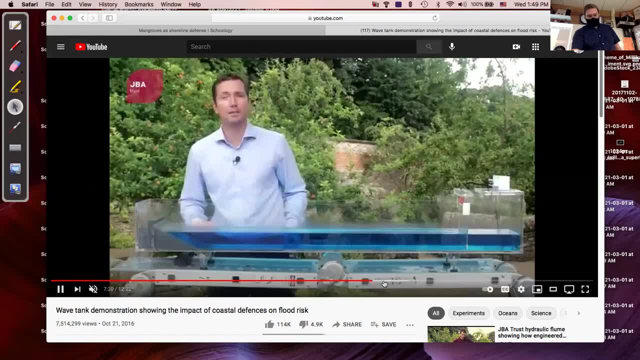 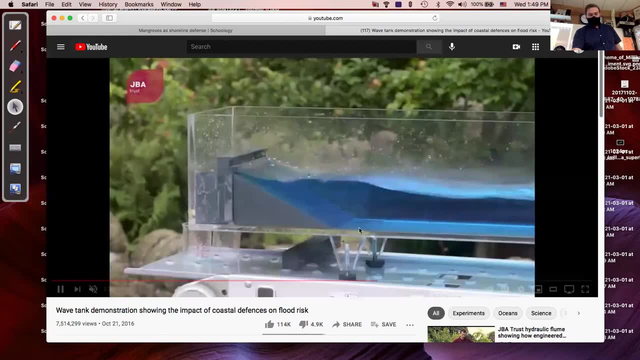 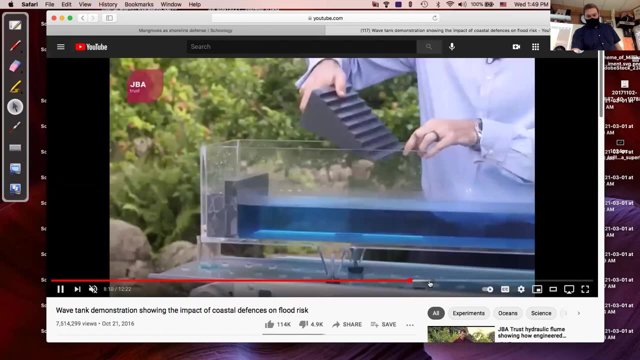 but they're pretty effective as well here. you'll see as it splashes, it'll uh bounce back toward the sea instead of bouncing straight up. but again, you can't have waves that are any taller than the top of the return, so it's relatively effective. other places they put in like a stair kind of. 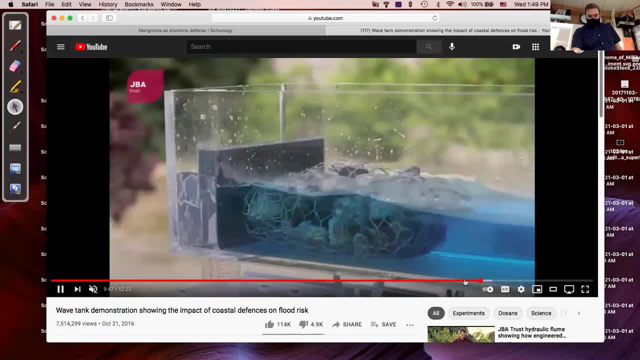 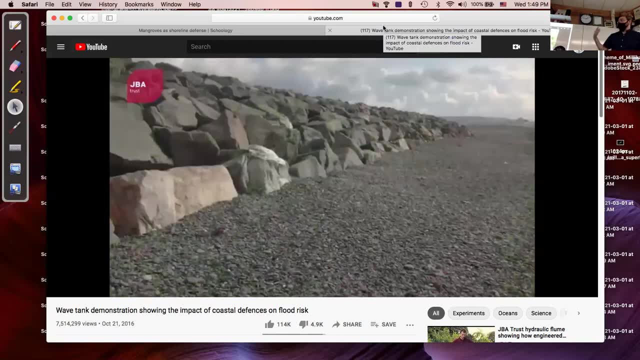 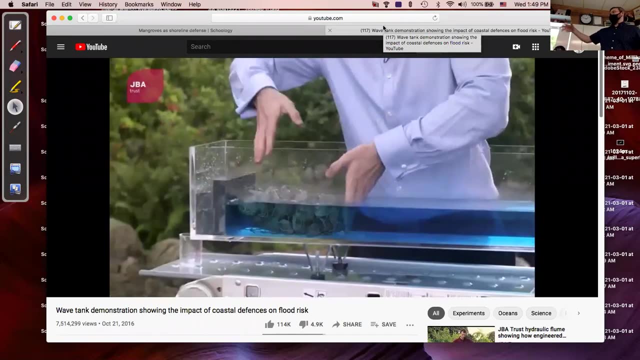 and uh, but the things that are very effective in this model as physical things are, you can make, you can have like a rock armor. rock armor is used around shorelines sometimes. it's a natural defense, so sometimes there's like uh, rocks that are outcroppings that are out in the water. 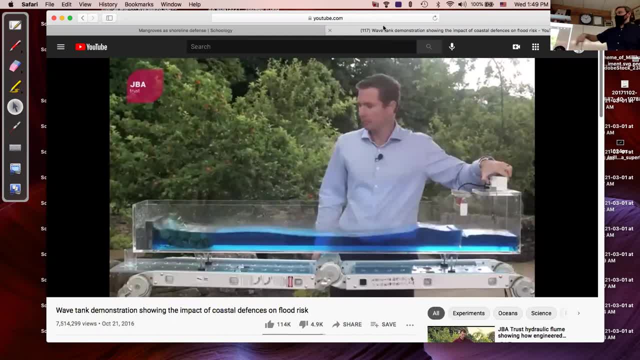 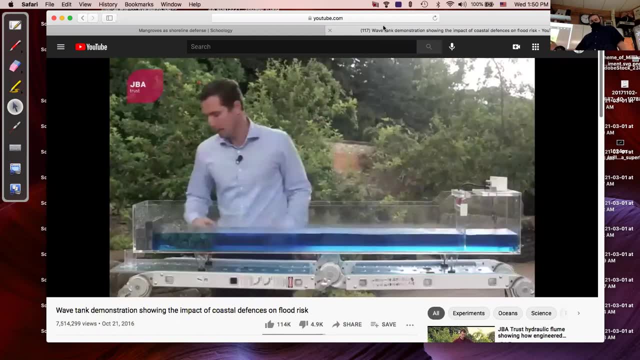 and the thing about the rocks is, as the wave energy hits the rocks, there's a lot of space between the rocks themselves and you get a really, really big reduction in the height of waves. so in some places they'll put baskets with uh rocks out in place and they're pretty good. 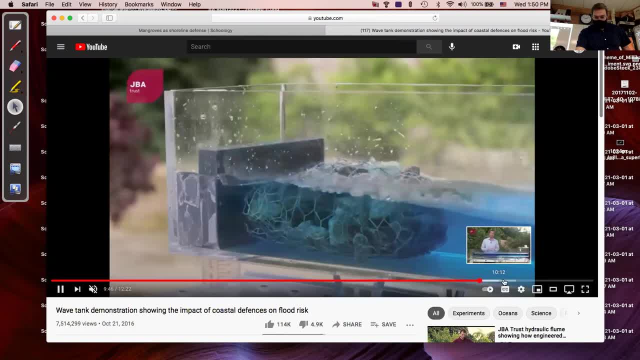 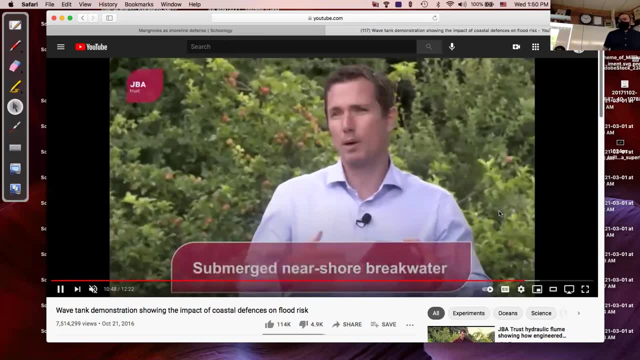 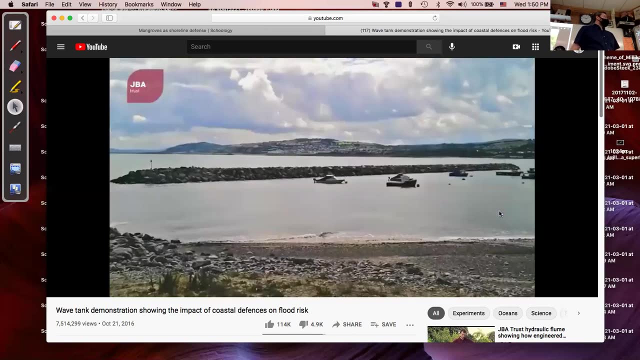 but another really effective thing to do is actually to put something further out into the water. that helps as a protective device. so here's like a shape that's like a- uh, like a pentagon shape, and it's not at the shore but a little bit further out. so they call them. 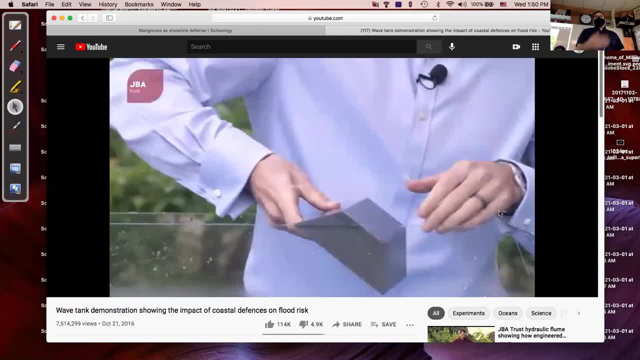 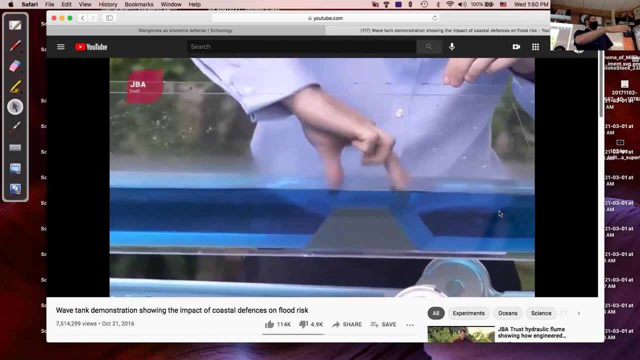 uh sea walls or break walls are oftentimes used to provide uh protection for marina and harbors. but one thing you'll see is that a lot of the wave energy when it hits that structure far offshore will bounce off the structure back out in open water and the height of the waves 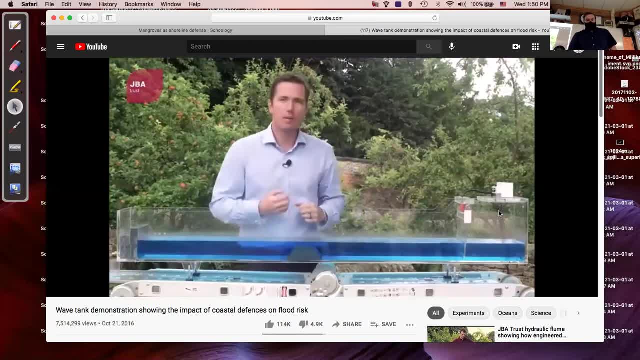 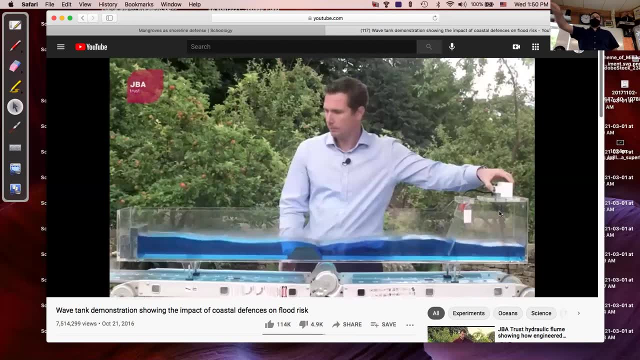 the left hand side of the structure is a whole lot smaller, so sometimes when you're at the beach you might go out in the water and then there's a sandbar that's out a ways, and that sandbar acts as a natural barrier, and sometimes for uh, coral, there are these barrier reefs, you know. barrier. 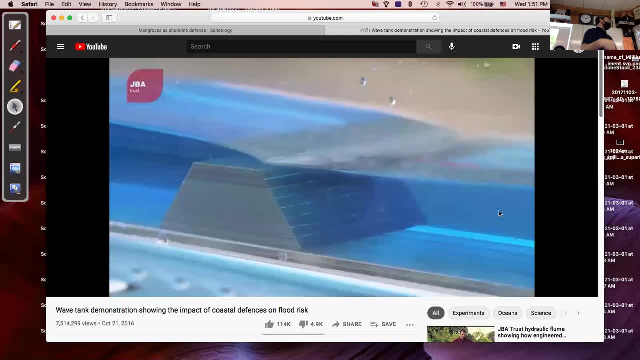 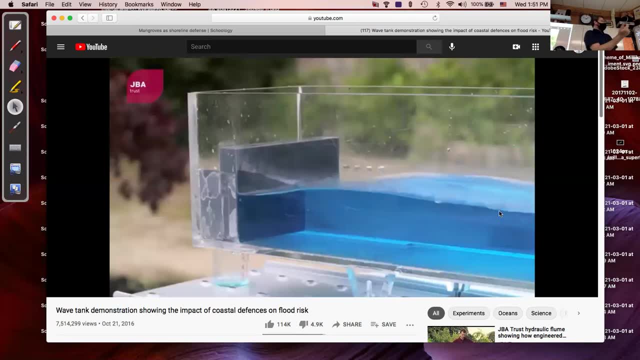 reefs might not be very far offshore, but they're parallel to the shore and they reduce the amount of wave energy. but here's, the waves hit that structure. some of the wave energy goes over the top, but a bunch of the wave energy bounces back. you see, here none of the wave energy goes over that original. 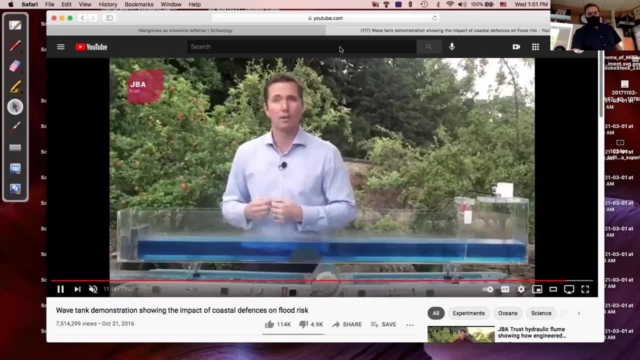 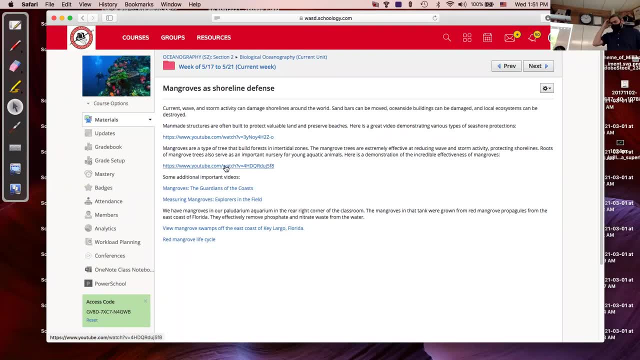 seawall that was initially present. so, besides physical structures that can help, uh is a very, very, very important way that coastlines are naturally defended, and that's with mangroves. so mangroves like a mangrove. mangrove is the name of a, you know, area of bushes and trees that are saltwater resistant. but then there's particular 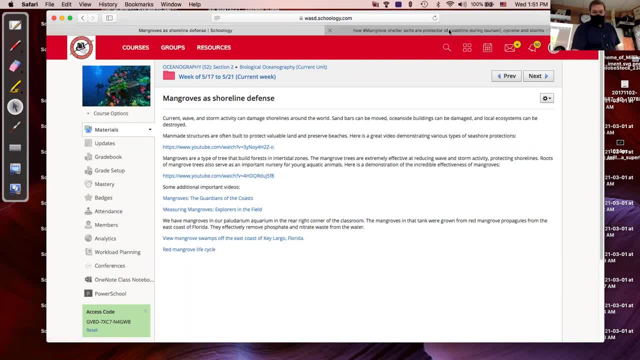 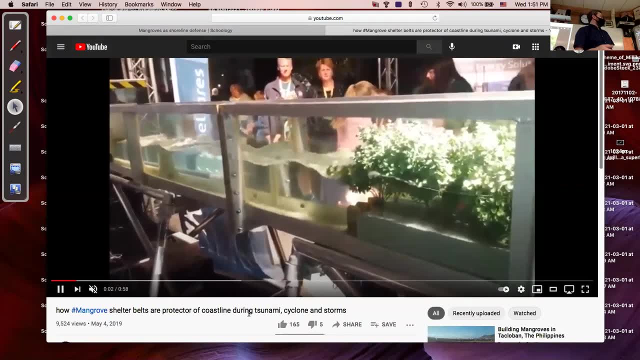 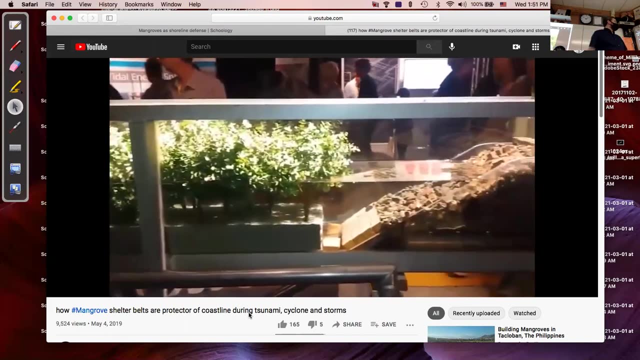 trees called mangrove trees, and this video here is a very, very excellent demonstration of the effectiveness of mangroves as a shoreline defense. so this is also has a wave generator. wave generators on the left make these pretty substantial waves. and then there's a little mangrove forest, and the mangrove forest is a little ways from the shore and nearly all the 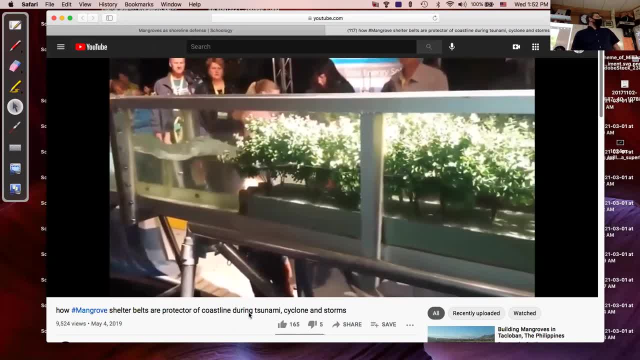 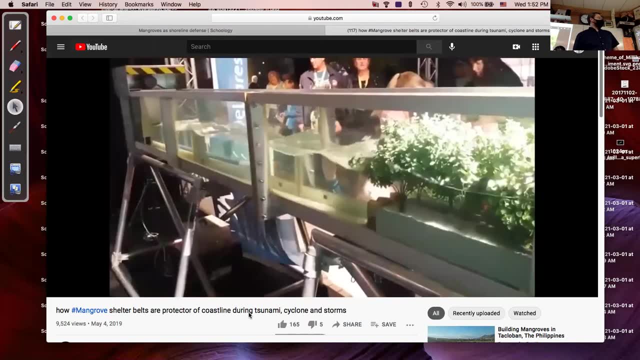 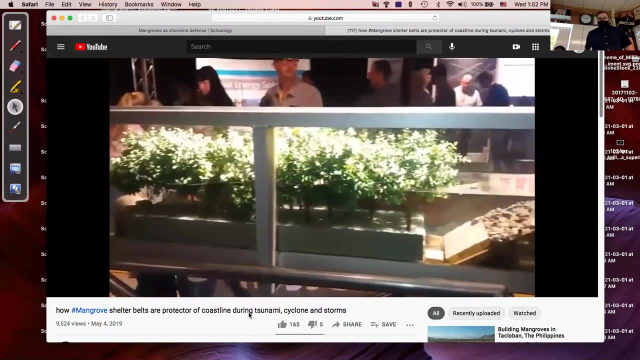 energy from those waves, which is pretty substantial, gets, uh really, killed by the mangrove trees and, as a result, the water level doesn't substantially change and you reduce the amount of erosion on on a coast or on the shore. so, uh, we have mangroves growing. there's two mangrove trees growing in the tank in the back. 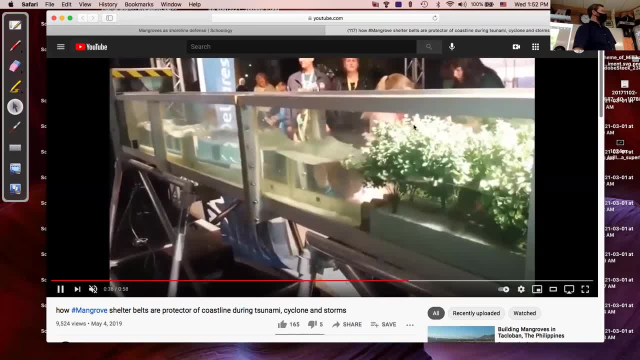 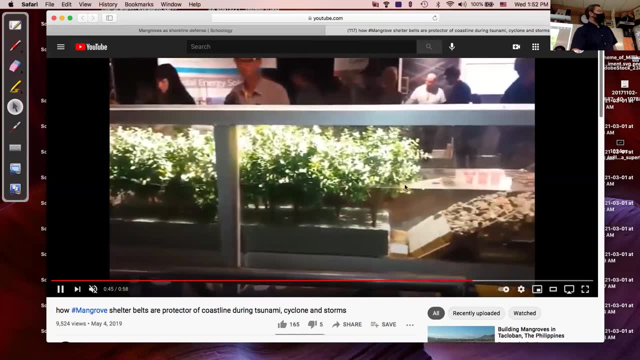 right corner of the room and it's kind of my goal to make that tank have a lot more mangroves in it as i get more and grow more. so they're kind of bushy like this and make that tank kind of like as a full-time tank. 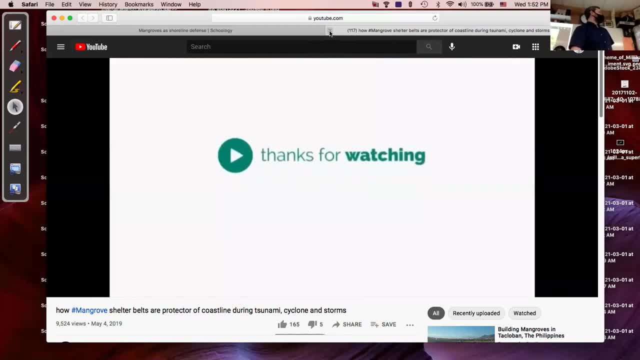 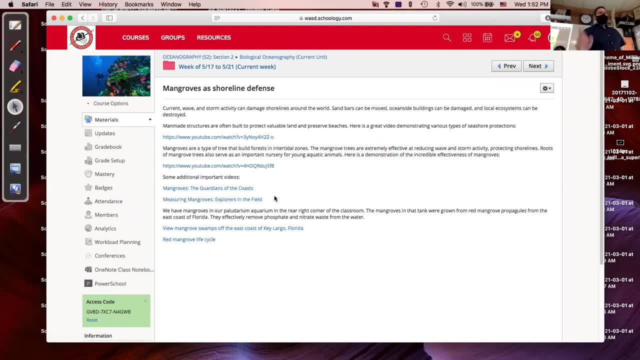 like as a full-time demonstration very similar to this one, but that's kind of like an ongoing problem. so the one here is the mangroves. regarding the post and measuring mangroves, explorers in the field, those are the ones i'm going to show like in class separately. so if 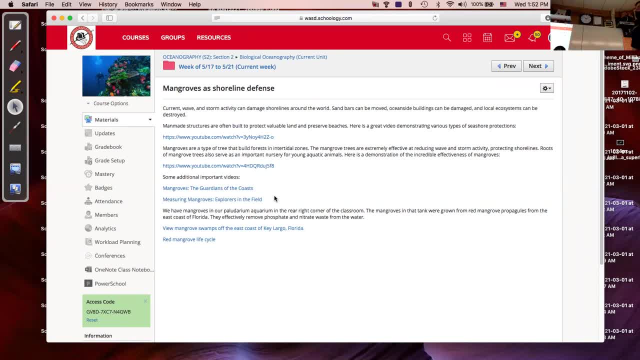 you're remote, it's best to watch them like on your own. these are only like a couple minutes long. uh, this one's pretty good, but then the second one is like a national geographic explorer series about, uh managing mangrove forests and their effectiveness for shoreline defense. 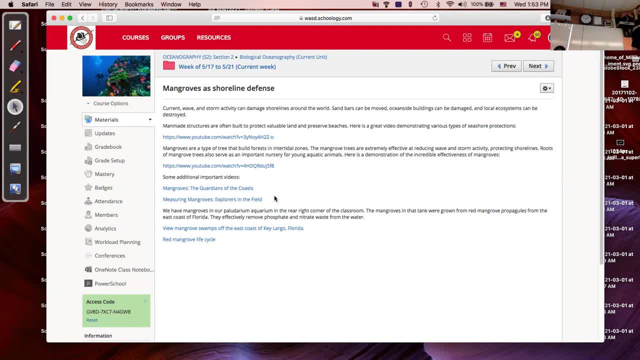 and you'll see there's other benefits. besides defending shorelines, mangroves are very critical homes for little fish and reducing sediment load and all kinds of different stuff. they also absorb a lot of nutrients to clean water up for like a sewage that runs offshore and things like that. 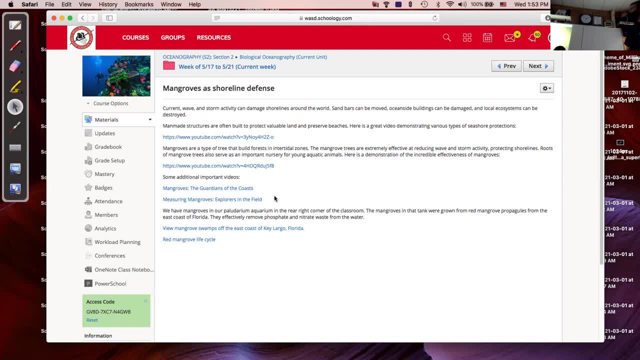 there it goes and i don't know what the answer is, but i have such a issues with the water problem. i've been eating it for like a year now, but the water is more intact now, so you don't really get to know anything about it yet. 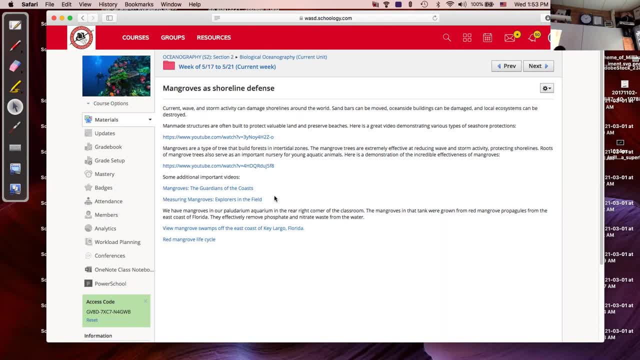 the mangrove forest is one of the most popular and delicious and most popular, and that's where we started, for our first arks was the ark at rioverland. on december 26 2004, disasters struck the coast of south india in the form of tsunami. 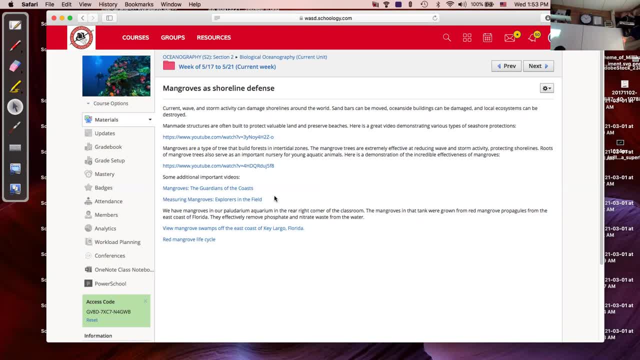 7 000 people lost their lives. the coasts were battered and ravaged beyond recognition by the surging sea. the aftertaste went breastfeeding to the coast of south india and seemingly killed a man from that beach. the coast was battered and ravaged beyond recognition by the surging sea. 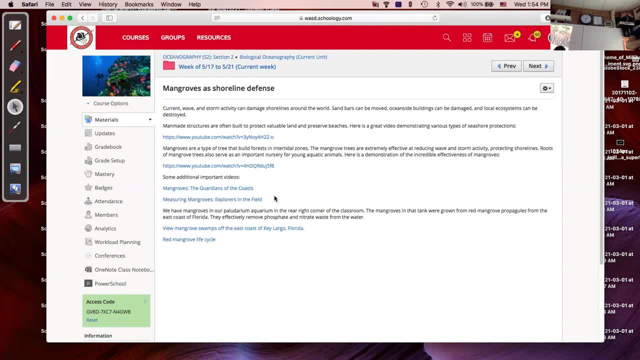 yet after this, we were able to see remains of mangroves and other species. the water was not released during the day because at the end, when we were there, we were able to see, Yet as the waves carved into the coasts of Tamil Nadu, Pichavaram, a stretch near Chidambaram. 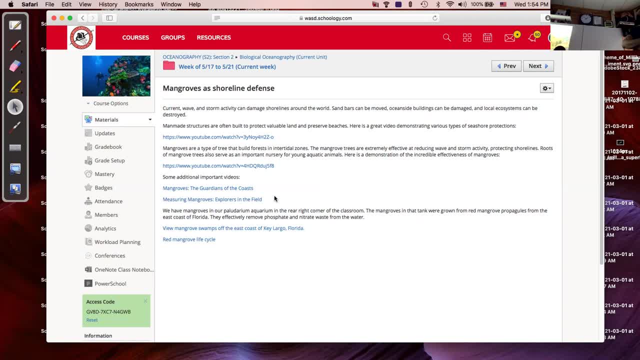 miraculously held against the rising seas and survived the catacomb. This virgin coast, undisturbed by man, was guarded by a unique ecosystem, which helped defuse the rage of the seas – the mangroves. Mangroves are clusters of diverse trees and shrubs that grow in tidal coasts. 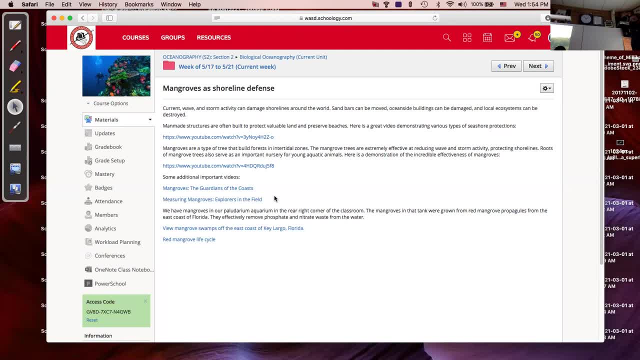 This tangle of groves which are salt-tolerant, stabilise the coastline, reduce erosion from storm surges, currents, waves and tides. The intricate root system of mangroves is home to a multitude of organisms. Sadly, more than half of the world's mangrove forests have been destroyed by flawed developmental. 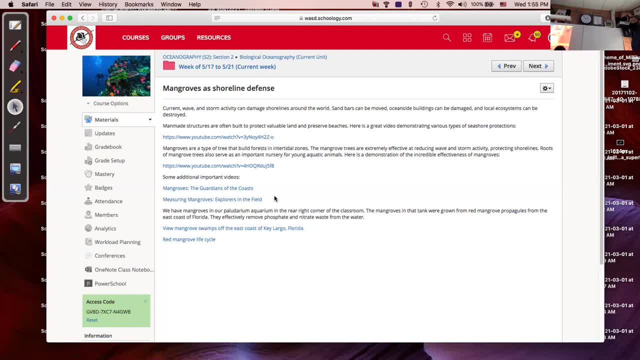 activities. Yet all is not lost – it is possible to reverse those damage and restore these vital biodiversity vaults. Small but significant equestrics are sprouting up, regenerating the forests of the seashores which is home to many. 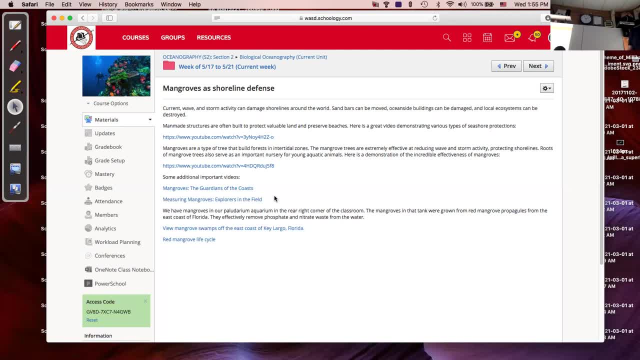 Here is a look at more complete of the role of the mangroves. Mangroves provide a huge amount of protection from a tsunami. Ancestrycom- Real rap. I'm on it like every day. Yeah, Yeah, Yeah. people have found family secrets, which is kind of awkward sometimes. 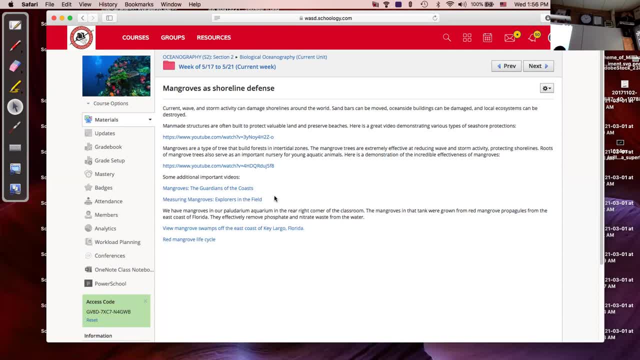 I know All right, so listen, you had to pick a color for a binder for each of these classes. I know, Stick with me. What would it be? You don't have to tell me why You can put an X down in one of those boxes. 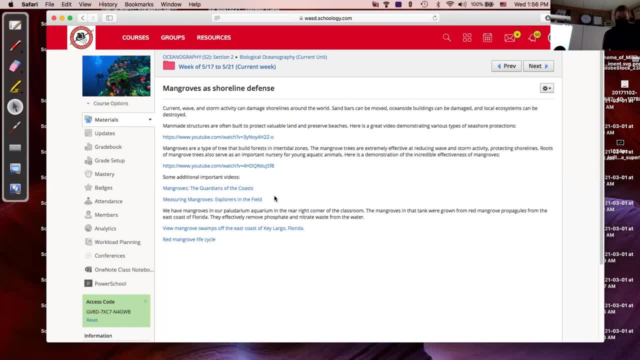 I don't know. What are you stating? I don't know. I'm telling you: We have to find out if there's an actual like correlation, and there is. There is 100%. If you say math is not blue, you're wrong. 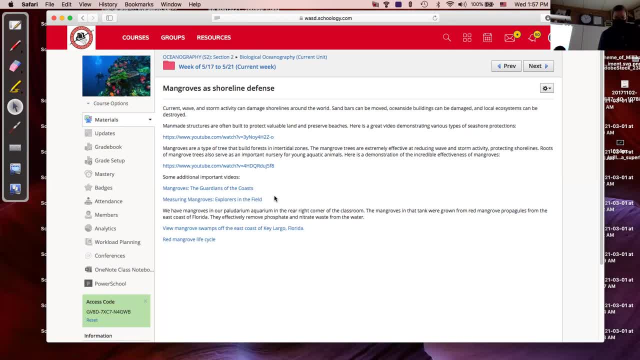 It is. I put red. It's either red or blue. Thank you See, Green, No question, No question Green. And I think yellow should be like blue. Yeah, Yellow should be blue, Yeah, Yeah. 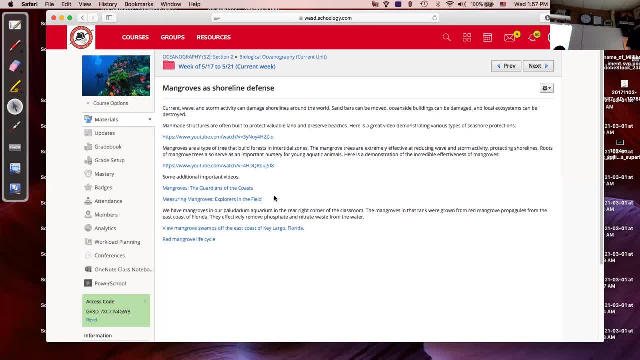 Thank you. I put green for science. That's cool. Yeah, Let's see. Oh yeah, So like people are finding people they didn't know, I have a close childhood friend who was adopted, but in a state. So every state adoption laws are different And in some states, like if the parents never want to be known, that's it. There's no way you, as an adoptee, could ever find out who your parents are. So they take an ancestry test and it will say: well, so it won't necessarily. So, like, if you give up a child for adoption, you don't want them to be found, don't take a DNA test, But if your brothers and sisters and aunts and uncles and parents do, then you know that's it. 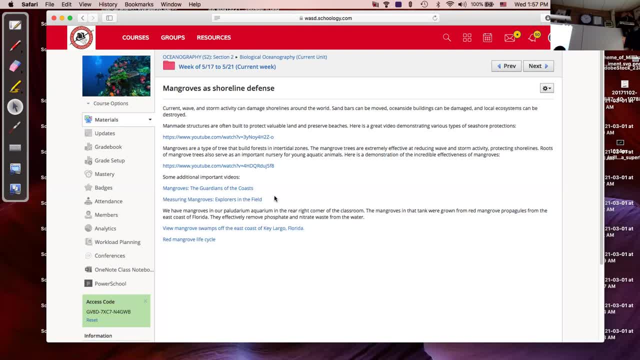 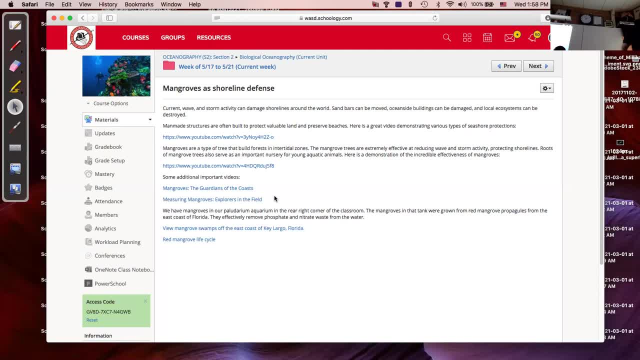 So it is actually a family secret, not a family secret, An unknown thing to our family. My fourth- like my fourth- paternal grandpa, like my last name, is not from a paternal line. It was my fourth great grandmother's name. 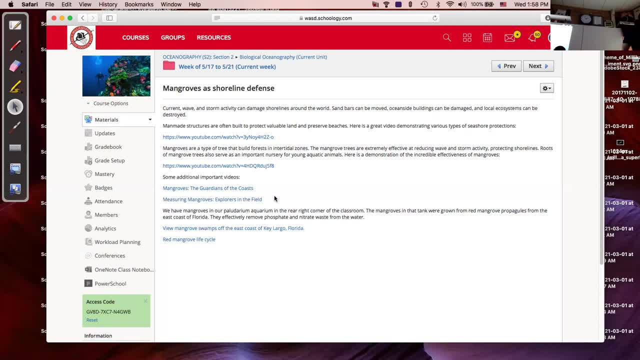 Class name, Right name. but she got like got knocked up by some guy and he took out- and it's not known to the family who it is, but i did a y dna so like, uh, what what's good is? because i'm looking for, like my father's. father's father's father. that is only passed down through the y chromosome, so what i need to do is figure out who that is and other men- so only men can take a y dna test and other men have, and i know that i am related by ydna to about 300 other men who have done it. but now the problem is: 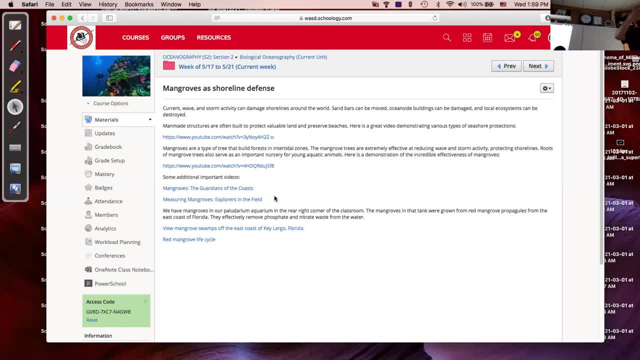 i need to actually build family trees for them and see where they come down to be in about the right geographic location, because you're like, i'm looking for a guy who is in central new york about 1850. you know what i mean. like, who is there? yeah, so the thing is, i know for about six or seven. 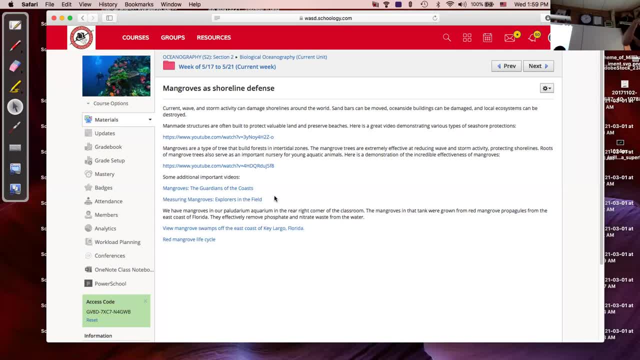 generations back, but most of those people were not. you can discount them because they're like they were all in california. so it's not them like why some dude can go from california in the 1850s to like new york, knock up some girl go back to la. it doesn't happen. no, it's like you're looking for people. are very mobile today, but in the 1850s people were not mobile. like you grew up on a farm and you may have only traveled 10 miles in your whole life. yeah, so like it's very, very hard in modern times to make those conclusions because you can just get 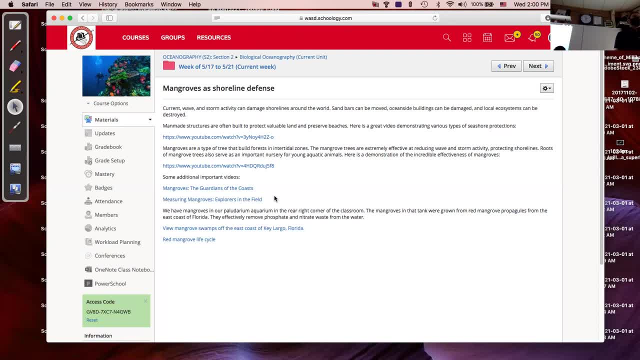 in a car and drive anywhere. people are very mobile, but it's much easier with older stuff, like you know. when you think about people moving state to state nowadays it's kind of no big deal, but if it's the 1700s or even earlier, you literally say goodbye and you will never. 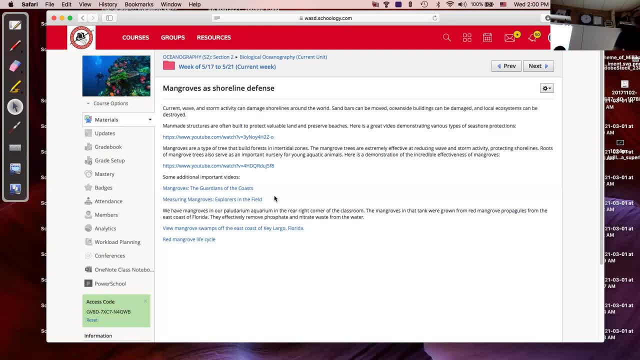 have a chance to say goodbye to the people you love, and you will never have a chance to say goodbye contact with those people again. you're going to a completely unknown place and you're devoting a huge portion of- like all- of your personal resource. you liquidate it, turn it into cash, get on a boat. 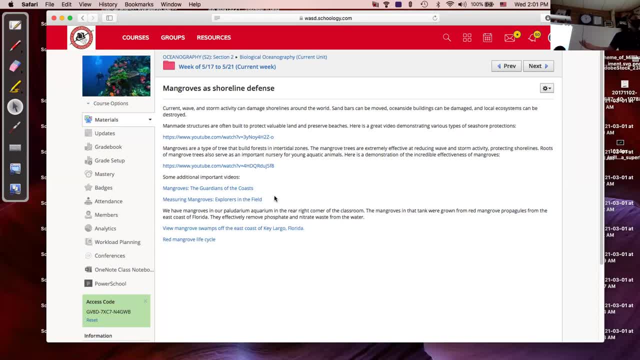 and show up somewhere you don't know. you don't know anybody there and you'll never see the people that communicate with them. yeah, so uh, when you think about the kind of migration and change that we've had back in the day, it's far more complicated in a lot of 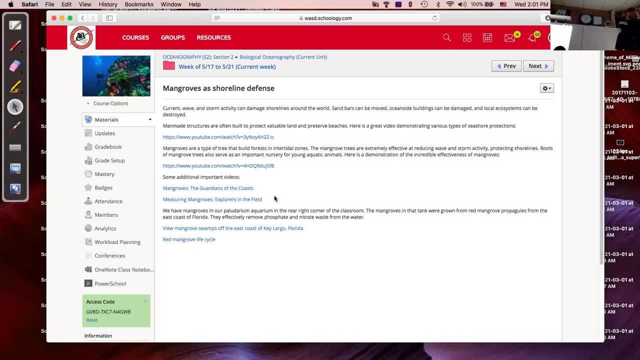 ways than this now, but it makes things, like on ancestry, pretty cool. there's also, uh like a family secret- i haven't quite uncovered yet, but it seems like like i just uncovered one. one of my great grandmothers also had another kid who probably was given up for adoption. because there's all these. 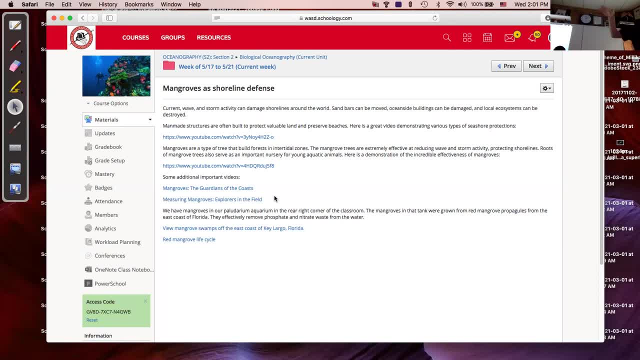 other people who are related to us through them, but it's not known to the family. so it's likely that, uh, my one great grandmother had a child who's probably given up for adoption. they have a whole bunch of kids but they don't know. they know that they're related to us but we don't know how. but somewhere there's- like someone who shows. 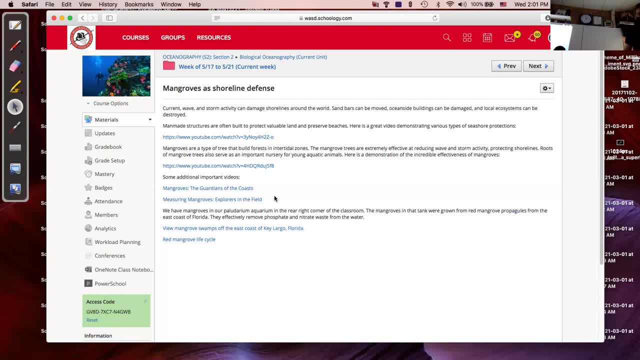 up my grandmother. she raised my aunt's daughter but it turns out that that daughter's daughter, yeah, she was right to think that the lady was her aunt, right? uh, i have a close friend here in town and she, who she thought, who she thought were her parents, were not her parents, they were grandparents. so i mean people in the family knew that's right. so you would be raised thinking it's your sister, it's really your mom and that way i mean the people know, like people in the family know, but they kind of keep it on the down low. you finally find out or you do ancestry. then you're like: oh, my sister's not. 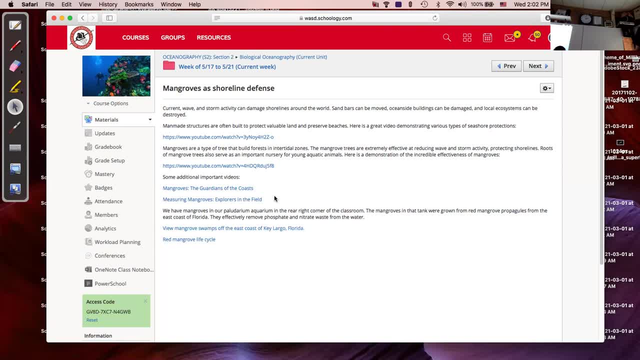 my sister, my sister's my mom. then you have to have those conversations like: hey, mom, so i did the dna test. uh-oh, yeah, but you know, like it is what it is, okay, this is pretty good. this is like: oh, it's just five minutes, but it's not quite five minutes to do the thing at the end. 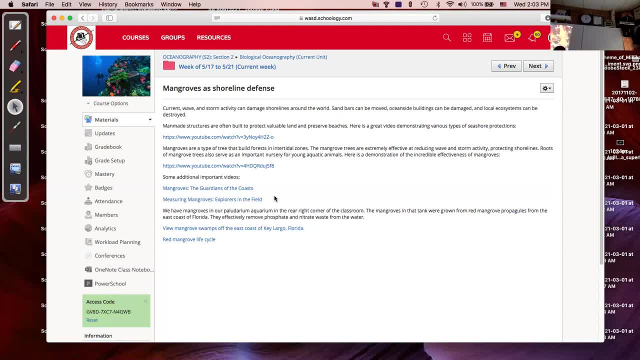 we jumped in the water and we saw many colorful fish and it was unbelievable. so since then, i want to do this and i wanted to to repeat that experience again. it wasn't until i turned 24, when i had the opportunity to travel all around the california peninsula, and that was the moment that i realized that i wanted to be an explorer. 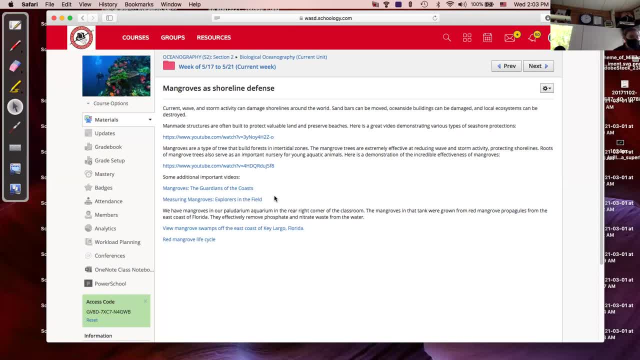 my name is octavia burton. i am a conservation biologist and a national geographic explorer. i am studying mangroves. mangroves are trees that live where the ocean meets the coast, and they are special because they grow in south water. here in mexico, i think, we have the most beautiful mangroves in all the time. 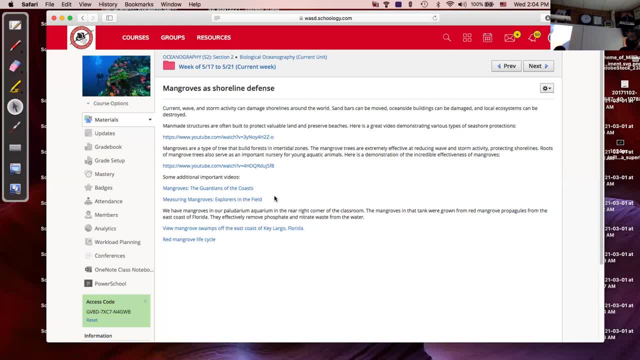 here in Mexico i think we have the most beautiful mangroves in all the time. they are the most beautiful mangroves in all the country, only beautiful. they provide a lot of economic benefits for coastal communities. roots coming to the water, they form a refuge for many, many baby pigs. 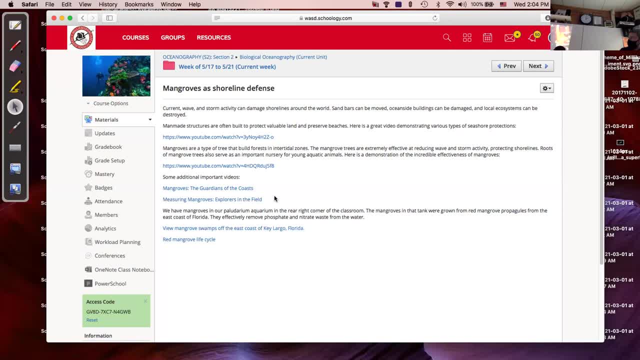 that they can live inside these roots like a nursery. it's like a playground for them. i just saw a big school of kidnappers and a lot of part of me. these juveniles only live here inside the mangrove and eventually, when they grow up, they will supply the fish markets here. 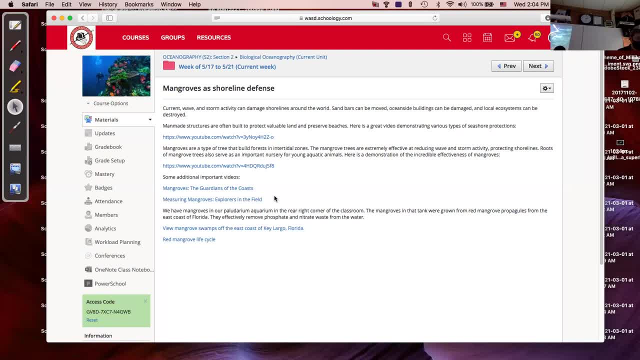 in the heart city. mangos protect coastal areas against hurricanes and erosion. they also filter water for many coastal towns. they also protect coastal areas against hurricanes and erosion. they also filter water for many coastal towns. they also filter water for many coastal towns. they also filter water for many coastal towns and provide essential habitat for many species. 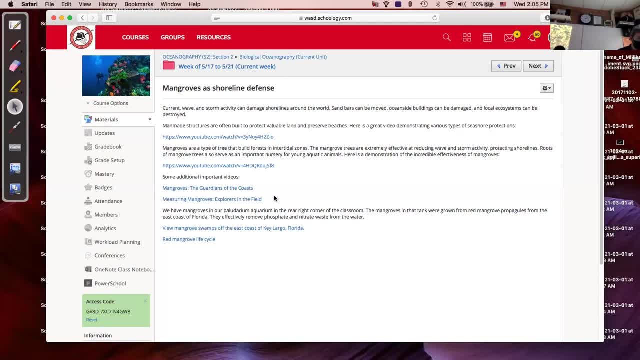 unfortunately, in the last 50 years, we have lost half of the mangroves worldwide, and this is because of agriculture, green farming, coastal development and pollution. the first step to help mangroves is to know how much mangrove we have in order to tackle this. 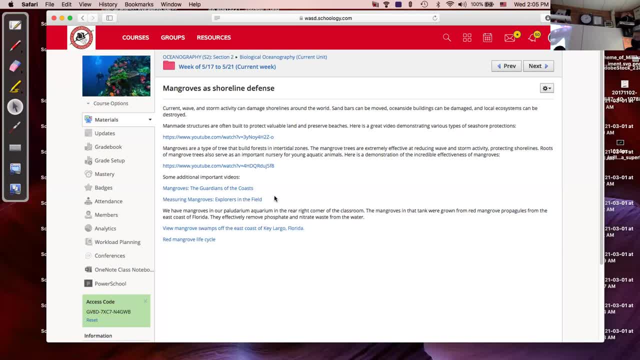 problem. the first step to help mangroves is to know how much mangrove we have. in order to tackle this problem, my research involves two techniques. one is counting everything that we have inside the mangrove roots, and the other branch of our research is to estimate the cover of mangroves. 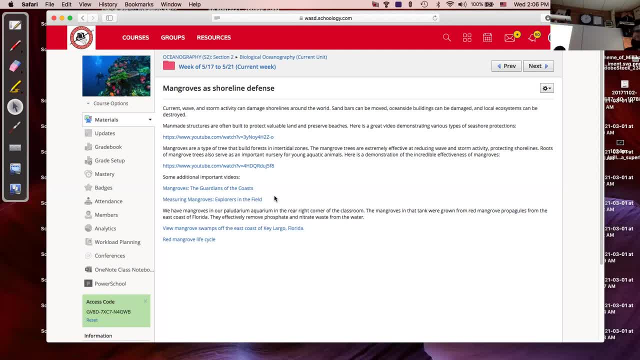 to estimate the amount of cover. we- we are using drones to estimate the amount of cover. we- we are using drones with drone technology. with drone technology, we are serving an area, Fly at different heights in 100 meters, we Largely not able to Souft. 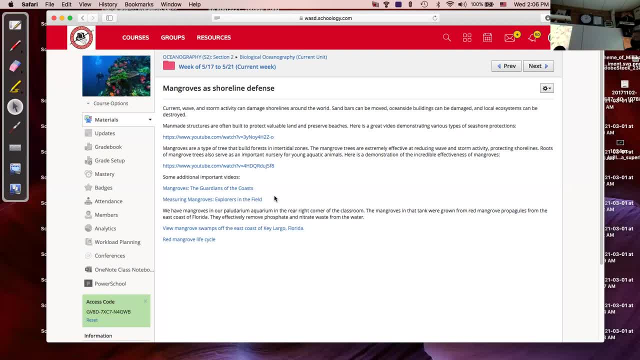 take a lot, take a lot of images. later we use all these images to create a composite image that is called ultramultiuse. later we use all these images to create a composite image that is called ultramultiuse. so you can use, or we can use, these images not only to estimate the area, also the volume of the points. 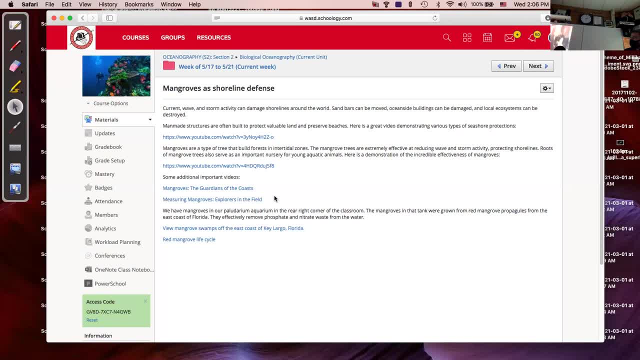 using all this data, now we know where are all these mangrove areas, how many animals live there, and we can set conservation priorities to protect this beautiful life. the involvement of local communities is essential to stop mangrove deforestation. if they understand that these roots protect their towns, create habitat for the fish that they sell. 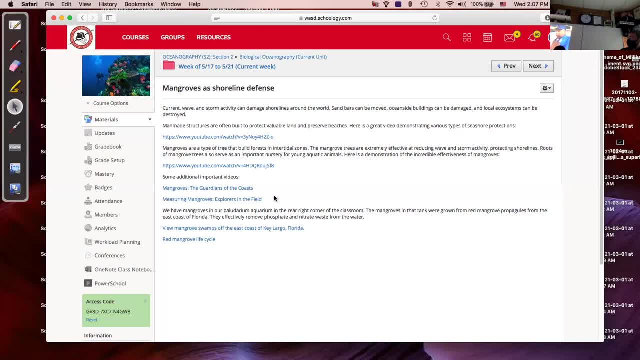 in the fish markets, we will have not only more mangrove in the future, we will have more economic benefits for them and for the rest of the country. mangrove represent a very, very tiny area in this planet, but they provide a huge amount of services for humans. 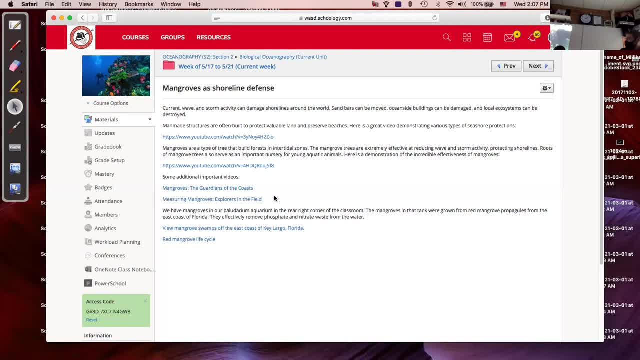 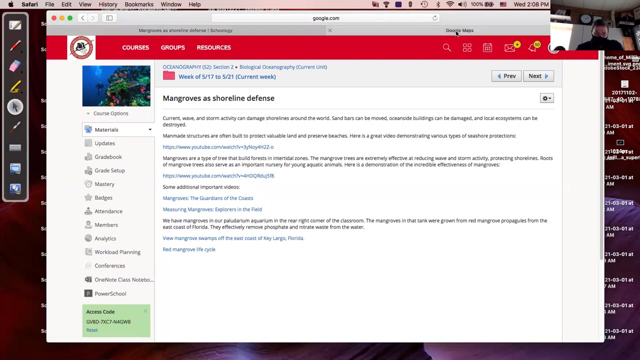 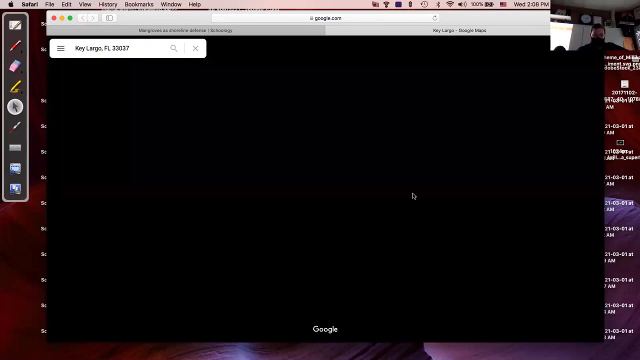 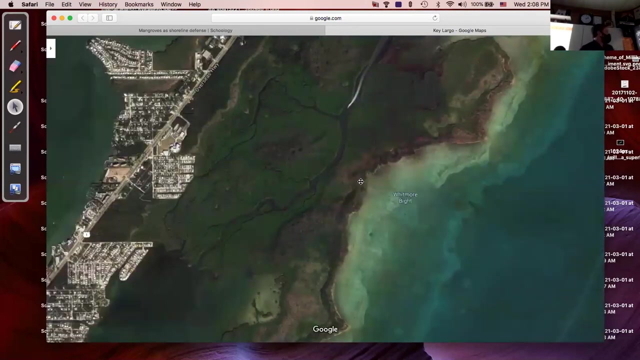 so we need to protect them for the future generations. so then, around the continental united states, we have mangrove forests and take it down here, okay. so if we go down to florida, there's a large key called key largo. it's the longest beach in the european sea. it's the longest beach in the european sea because the lake is the longest boundary. 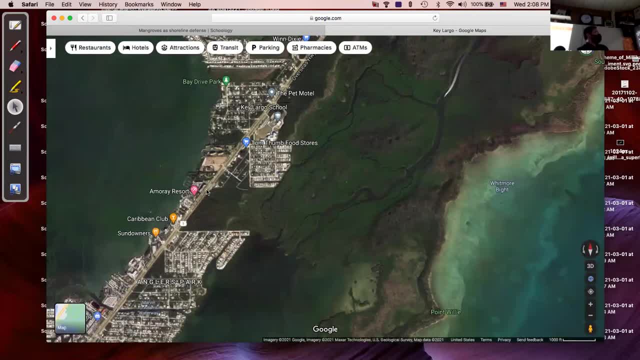 of the keys and on the uh west side of north side of key largo it's open bay, but on the east side here these are all mangrove swamp and actually you can see a boat traveling down through a river that's in the mangrove forest itself. so there's a housing development here and then there's mangroves. 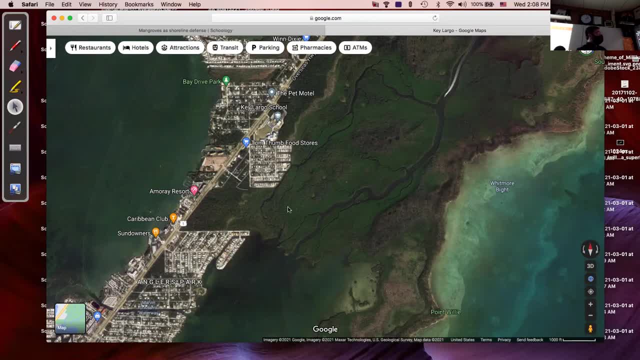 all the way out to where. uh, so it's water all the way from here out to here. but this is all a mangrove forest, the mangrove swamp, so you can't walk across land. instead, the mangrove tendrils extend down to the bottom and then, uh, there's some coral. that's out here the reason. 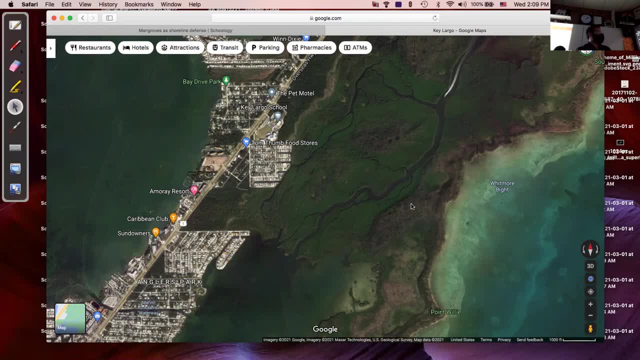 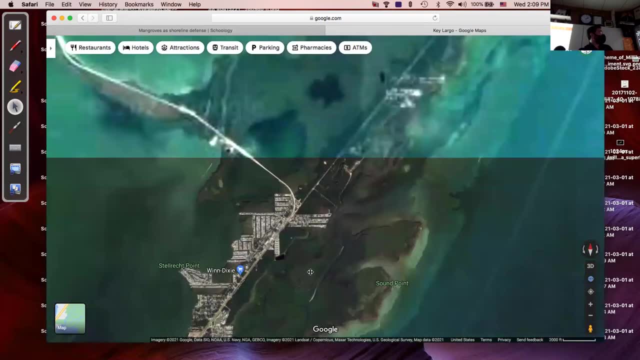 why you might want to get rid of all the mangroves is because then you get a nice like shoreline so you can see out to the ocean. the mangroves sort of like block of view. but in this part of key largo there's this huge mangrove forest toward the north. those mangroves don't. 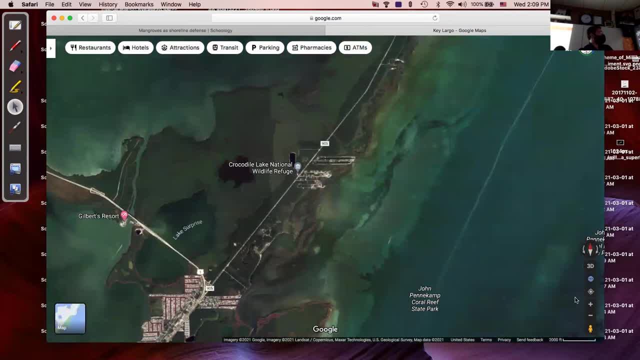 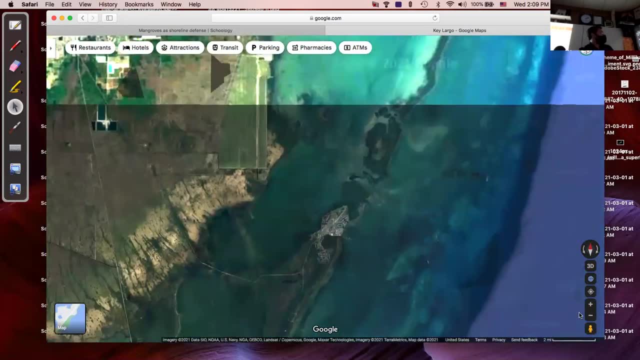 exist. so here's some people and there's like kind of no mangroves, but the mangroves themselves offer a huge amount of protection up along the coast of florida. um, if you would go up to like the south beach, you can see like a huge amount of protection up along the coast of florida. 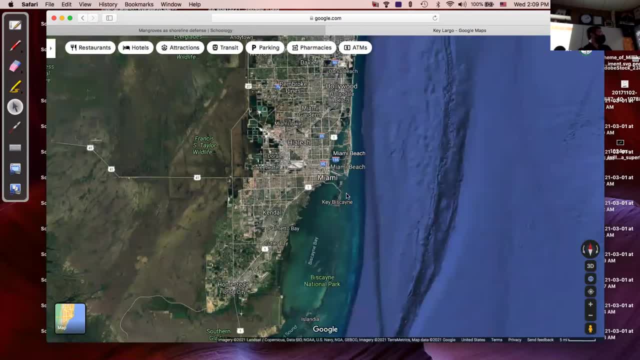 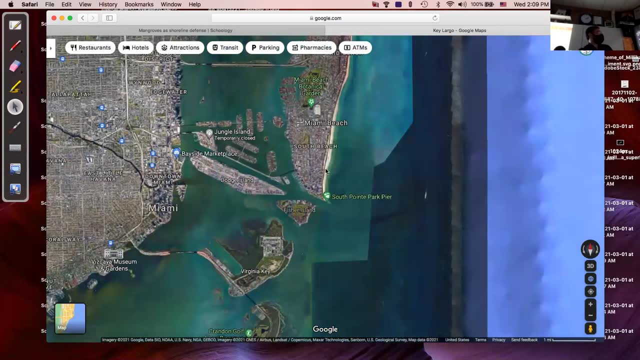 so you can see like a huge amount of protection up along the coast of florida. so here's like the city of miami, and where miami beach is and key biscayne, there are no mangroves, instead it's just- uh, you know, this is like, this is south beach when you think of like the beach in. 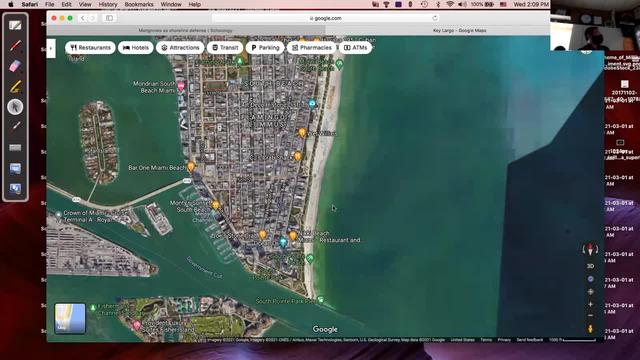 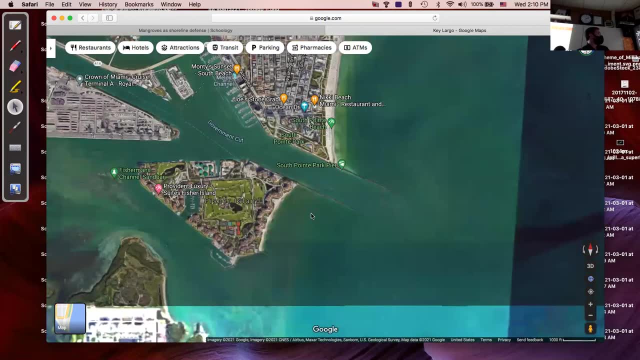 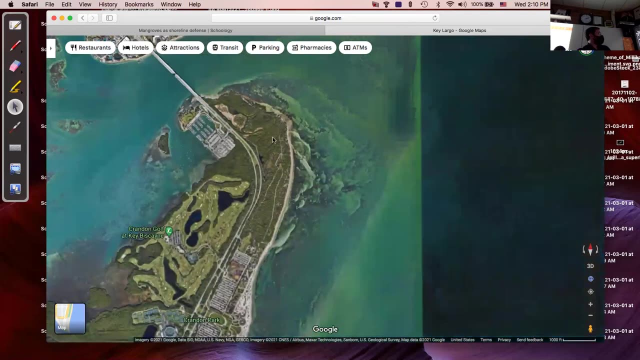 miami and south beach. this is south beach miami. there's no protection here on the coast, so storm surge that comes in from uh hurricanes, large wind and wave activity directly impacts the coast. so but if you go just a little further south- uh down to like virginia key and stuff- there are mangrove swamps here along this. 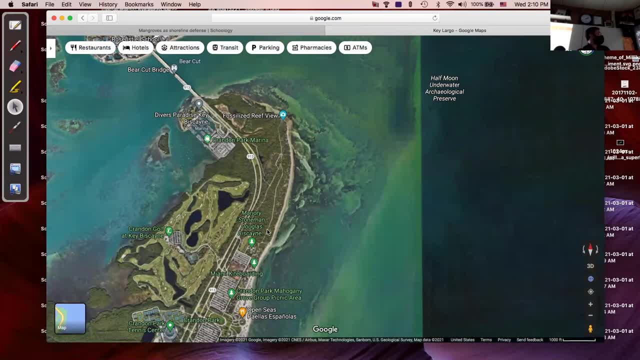 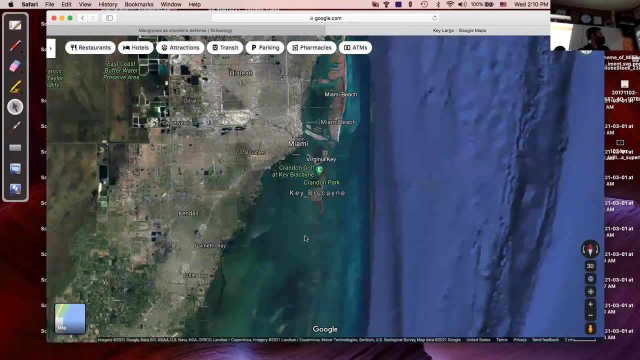 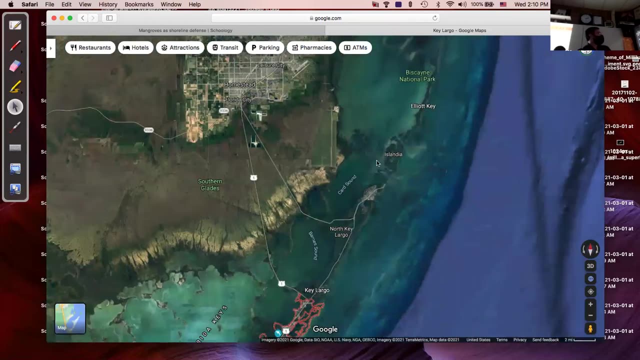 shore, so this shore is more well protected by mangroves than uh up in miami itself. uh, i gotta go further down, like down into here. so all along here there are, there are, uh, there are those mangroves. you might not know this, i don't know if you know, but if you can go, 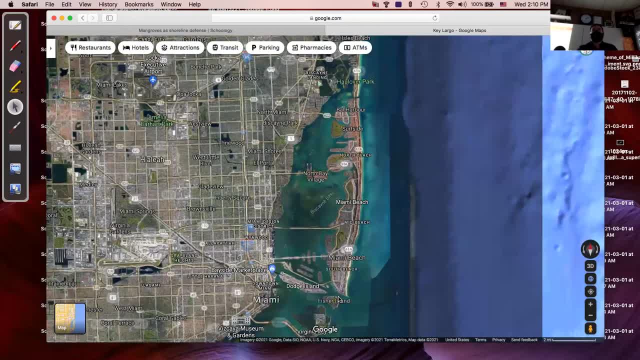 up into the ocean and you can get the water from this tip of miami beach all the way up to boston and never have to go out into the ocean, because there's a thing called the intracoastal waterway. i don't know if you've ever heard of that, but for instance- uh, oh, i showed you. 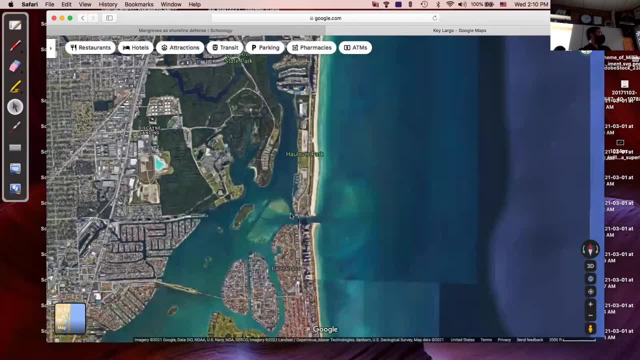 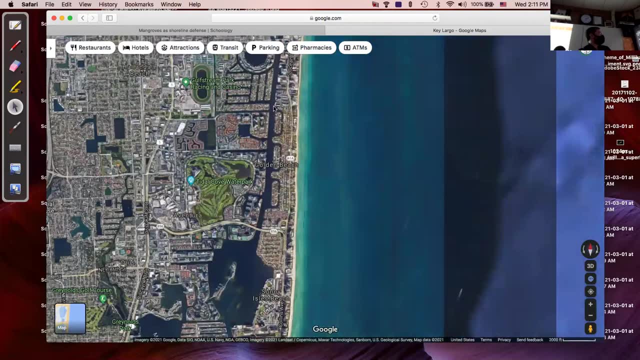 this video of fall over inlet, which is this little inlet here you can call: go into fall over inlet and then if you look up, if you look on this map all the way up through here, and there's this, there's this uh waterway that goes north like this. 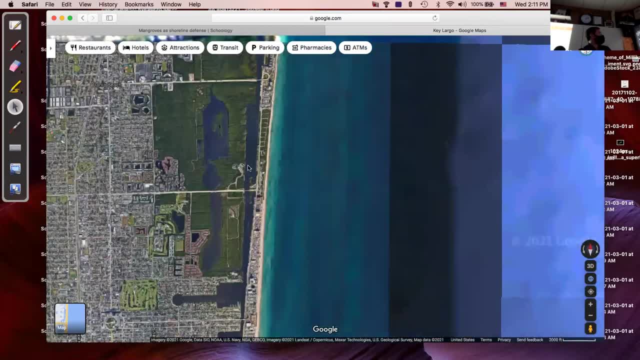 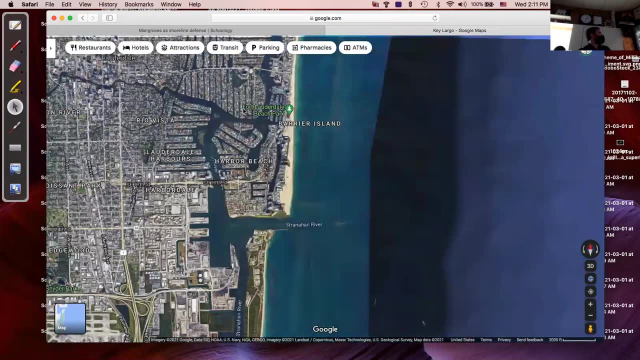 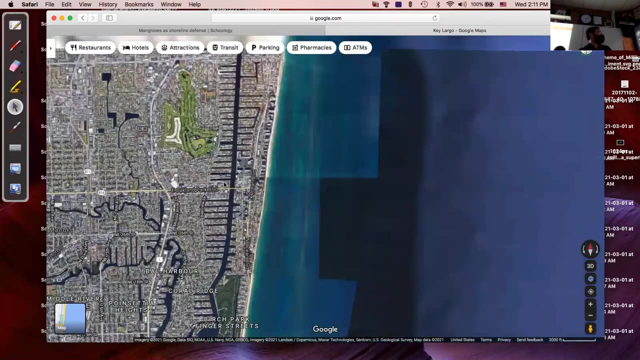 up along north and just keeps on going. we've only gone like about three miles so far, but this waterway, here it's. this river extends all the way up to boston, massachusetts. you don't have to actually go out into the ocean. this intercoastal waterway is used for to transport uh materials. 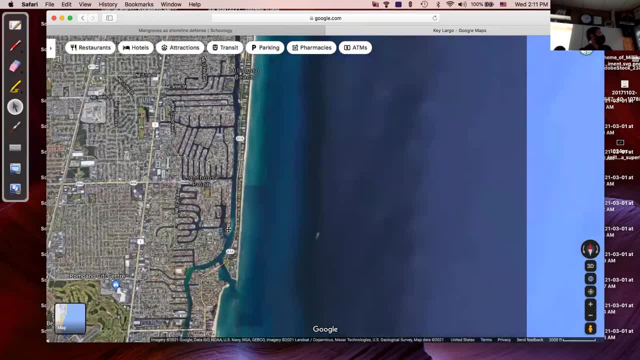 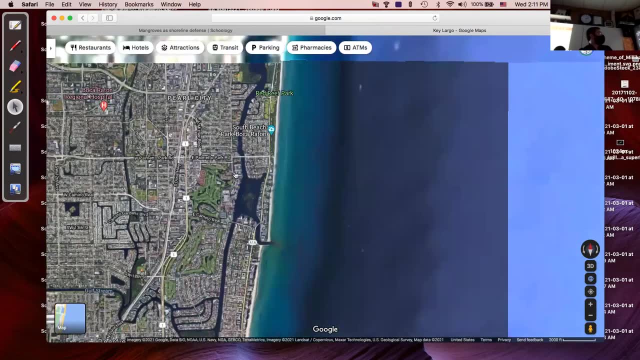 but it's also used by pleasure boaters and the that waterway is protected by either, in some places mangrove swamps, in some places, uh, another shore which is off the shore here. so we just kind of keep on going. you can follow this waterway all the way up. 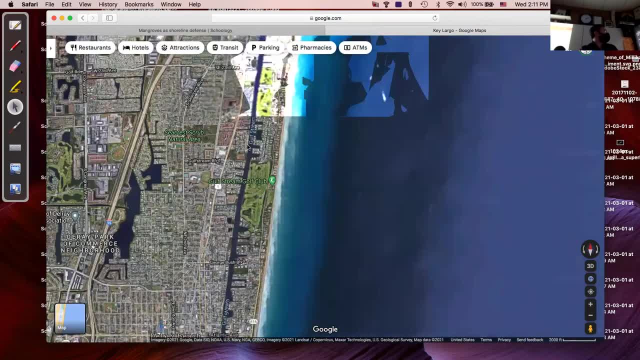 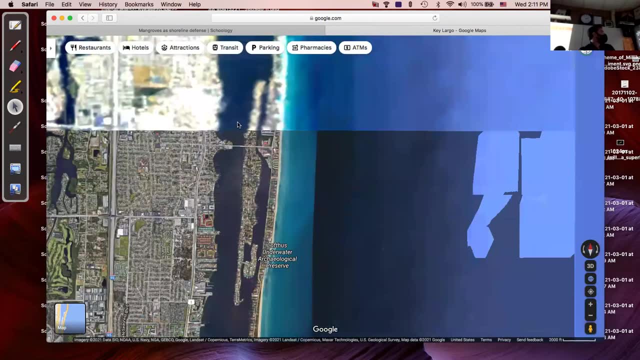 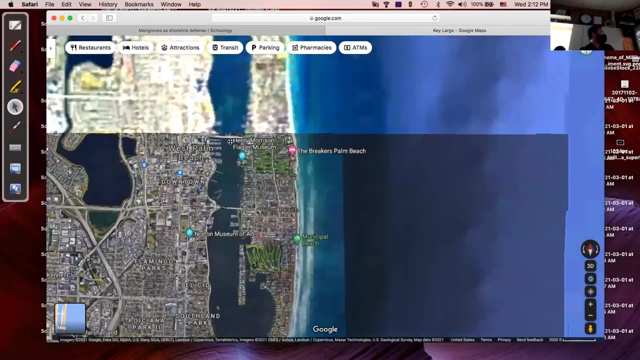 uh, it's about 3 000 miles, so it's really like a uh. in a lot of places it's a canal, in other places it shares a river. it just kind of keeps on going. some places it's wide, some places it's narrow, but it's. people call it the intercoastal, but it's the intercoastal waterway. 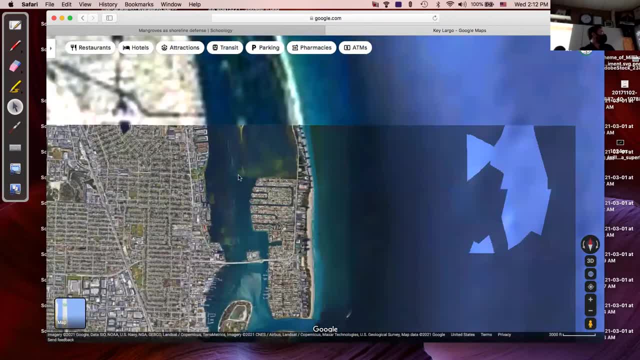 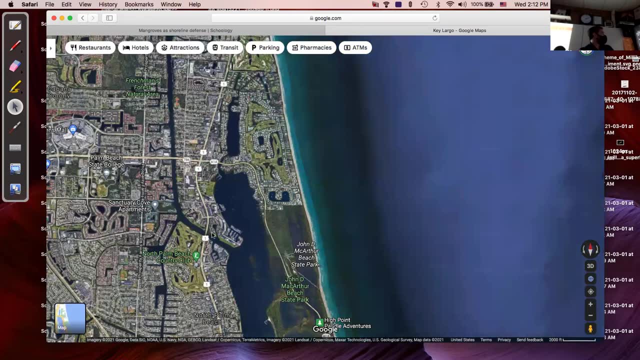 it just keeps on going and going and going. there's always land to the east and land to the west, and it just keeps on running. here's a place where there's like, uh oh, it splits. you have to go under this bridge and then up through here, and now it continues like this. so up in here there's a little. 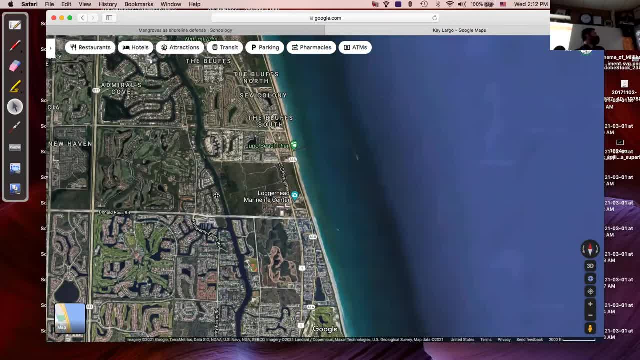 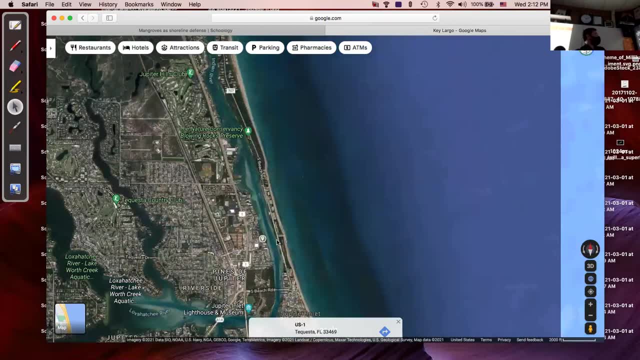 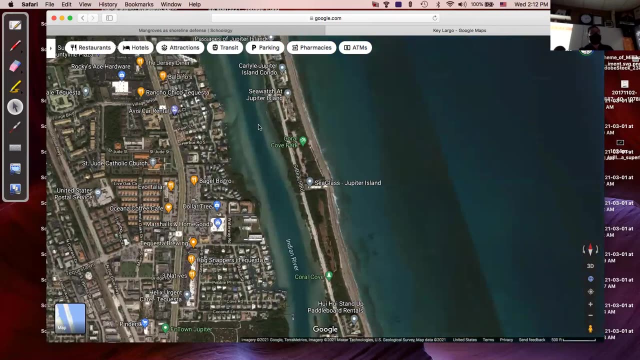 bit less development and these could be mangroves in this area here and just keep on going. then it goes over this part and, uh, this place it's dredged. you can see the sand and how it's shallow. so it's not just a plain sand, but it's a very, very dense and very, very dense water. so we're here in shallow. 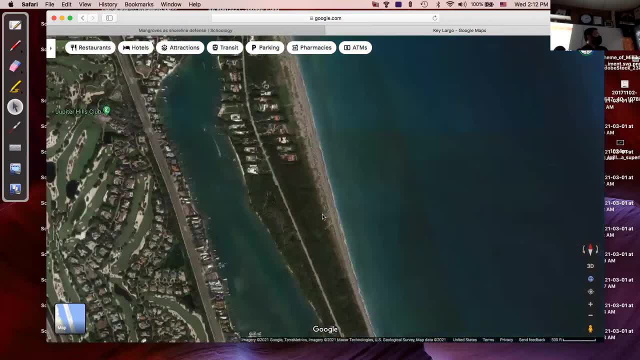 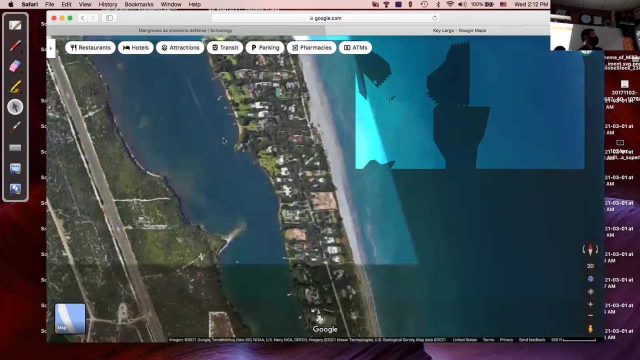 water here. this is intentionally dredged, so you go in with ships and dredge the, dredge it down so that you end up with a great enough depth. so here this coast, this uh barrier, provides uh storm protection to uh things on this side, but we're still in the indian river. some of these rivers aren't really. 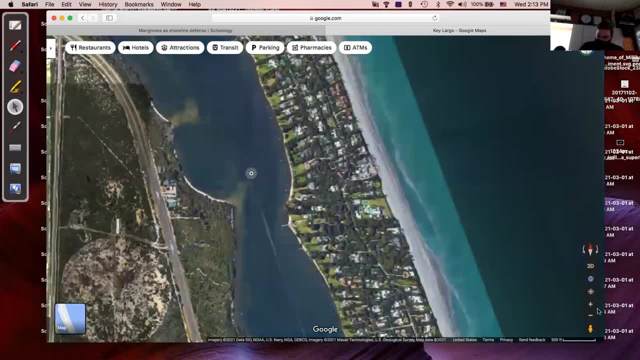 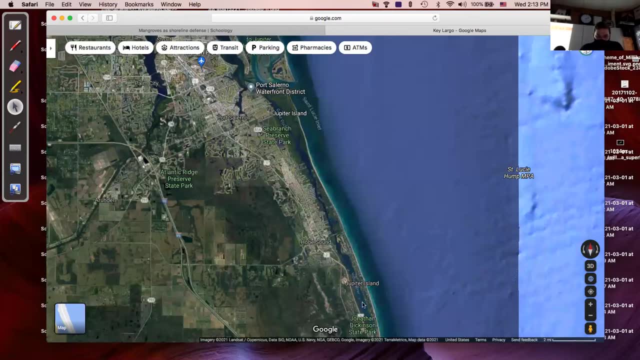 true rivers that are man, that are man or natural rivers and man-made waterways. they're given the coast and in some places along the coast it's- uh, protected by mangroves. you can see it run up along this and it keeps going up through here. so basically, you don't have to go out into the. 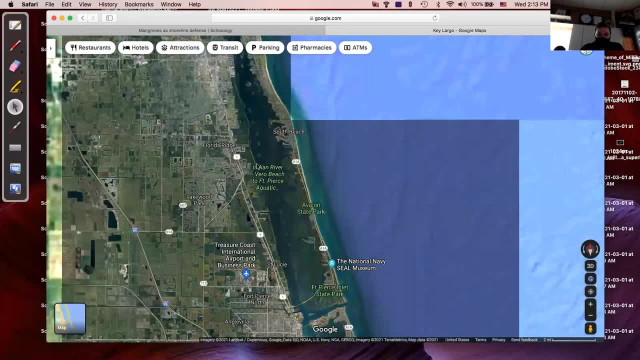 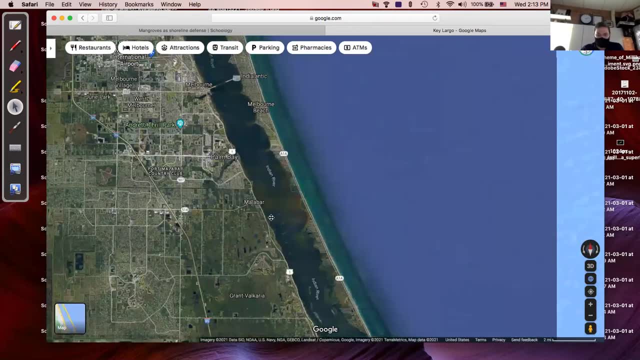 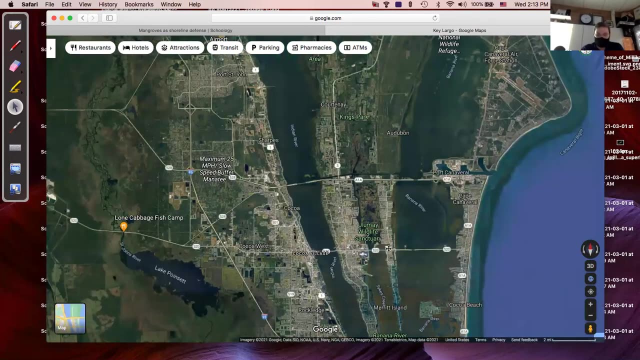 ocean to run the whole way up, and it's a very popular thing for uh pleasure boaters to run the intercoastal waterway. you can fish in it, um, but it you're generally protected the whole way from uh any kind of- like you know, heavy water that's out there. even here you can see that. 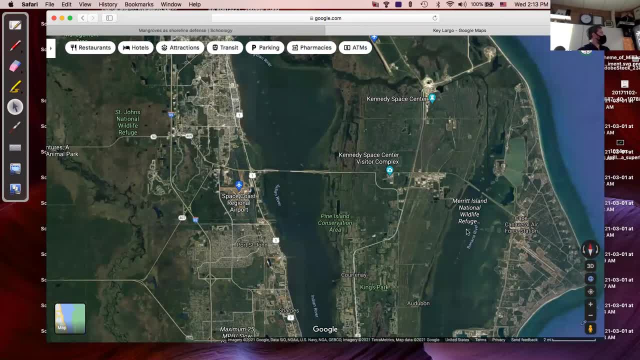 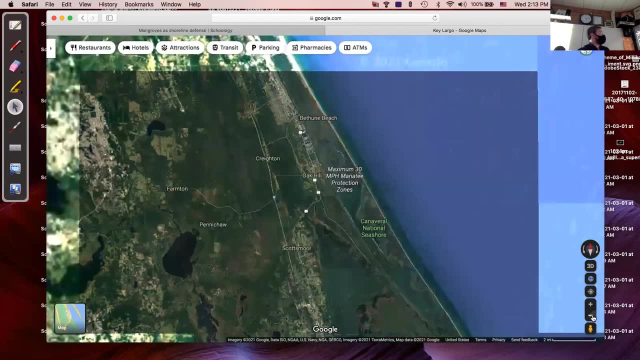 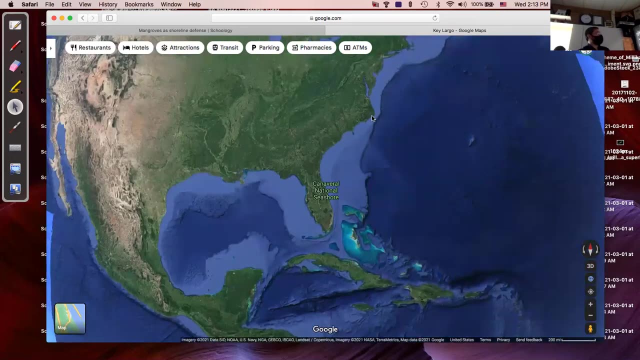 there's like these. these might be tie-ups along here and here, but it could be dreadful, but that waterway just goes. it's amazing. it's. one of the things that people don't know about our country is that you can get get into miami and run all the way up continuously, i know to um north carolina. 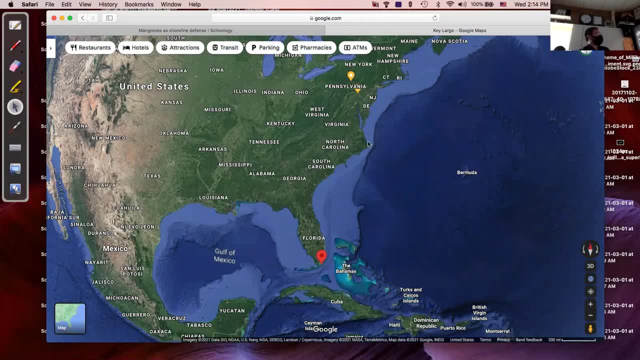 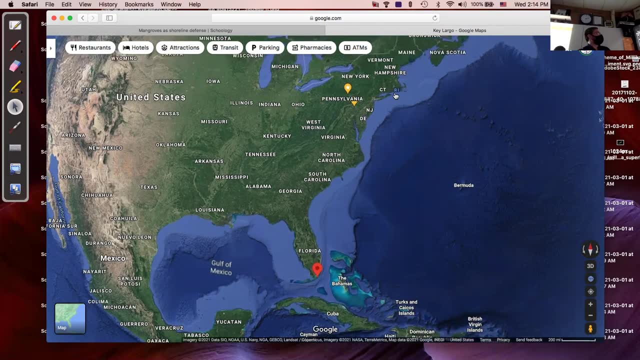 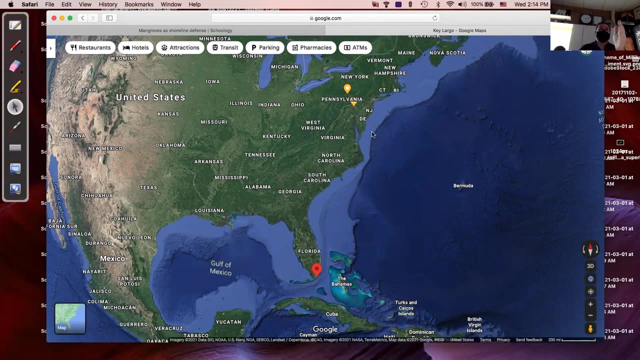 it's completely inland. in some places you have to get out and be along the shore and be in, like the chesapeake bay and whatnot, but basically you can get all the way from boston down to miami staying inland, but in a boat the whole way. that does not exist on the west coast at all. there's no. 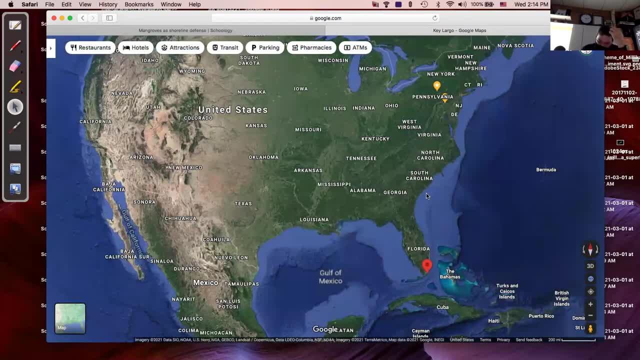 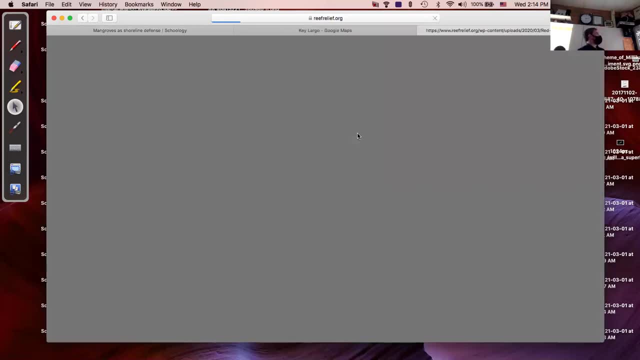 inland waterway on the west coast, but those east coast waterway protections are sometimes, uh, sometimes- a mangroves. all right, so here's the thing about how the life cycle works. uh, back in the tank too, you'll see these things called propagules. the propagules are like seeds. 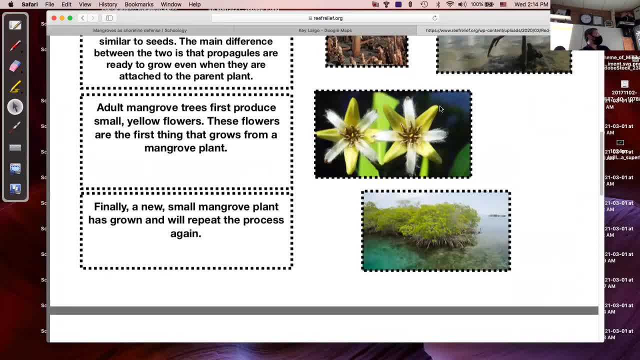 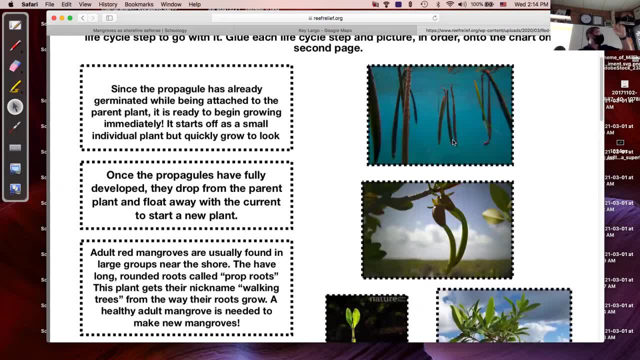 as the trees grow. uh, the trees drop the propagules off and the propagules kind of float in the water and they float along until they reach somewhere where the water is like shallow and kind of muddy and the broad bottom of the property will stick in the mud. 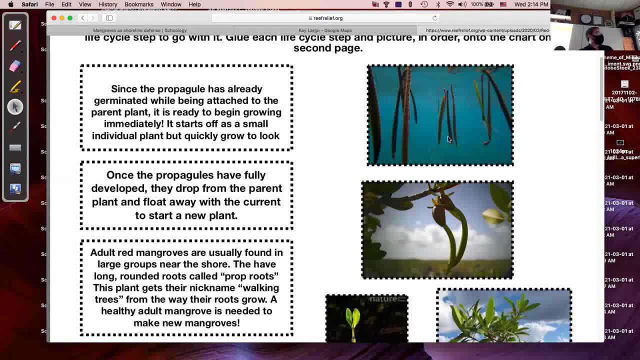 but uh, the mangrove trees continuously produce these seeds or mangrove propagules, and if you go down to florida you might see them washed up on the beach all kinds of different places. they're like about 10 inches long. they look like a stick, but they're really just like a seed. and then uh, 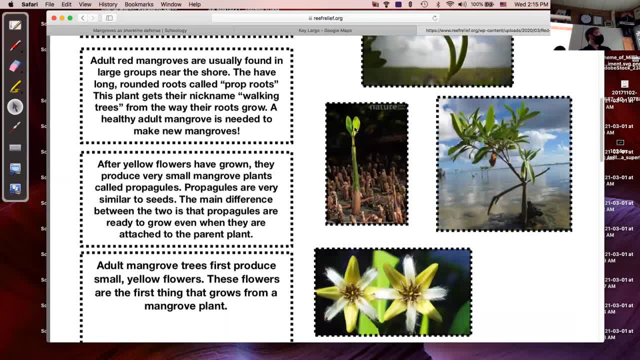 those things will stick in the mud, and whenever they stick in the mud vertically, then they'll begin to sprout. they take nutrients from, uh, whatever substrate they're stuck in, continue to grow up, develop leaves and then- uh, you know, the leaves undergo photosynthesis with energy from the sun and carbon dioxide from the air, and water from the water. most plants can't. 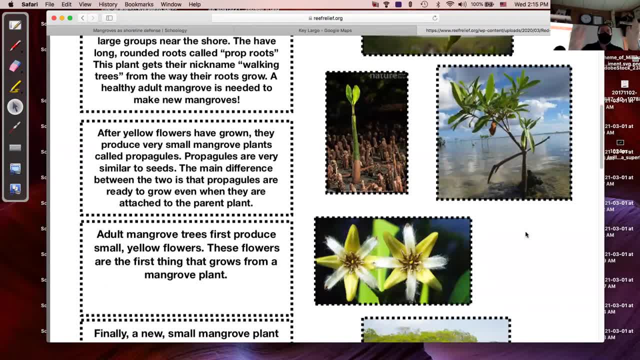 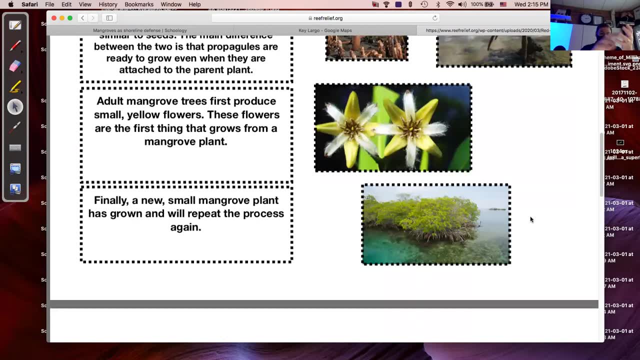 deal with salt water, like if you go, if you have plants or have a garden and you put salt water on it, you'll kill your plants most. all plants cannot deal with salt water. uh, with a rare exception are mangrove trees, and the trick with mangrove trees is they do one of two things. there's they're either. 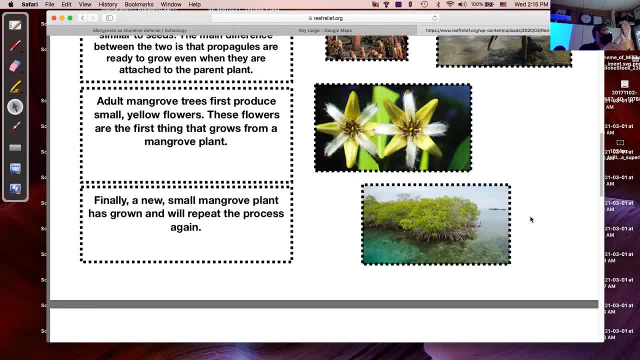 salt excluders or salt excreters. so salt excluders are uh mangroves that use a uh membrane to allow to pass into the cells- the mangroves we have in the back of the room. they're called salt excreters. so one of the things i got to do with those mangroves that grow in the thing back there- 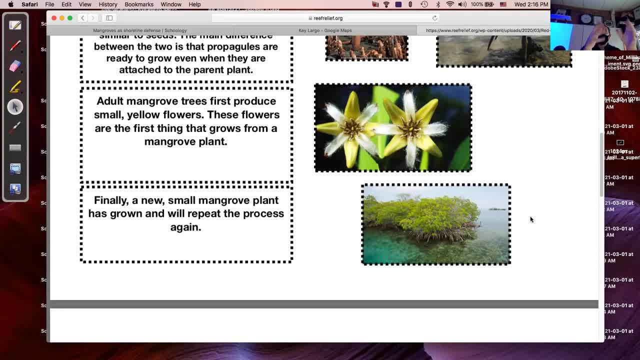 and you'll see this on the on the leaves and on the stem of the plant is there'll be salt like stuck on the leaves and on the uh wall of the plant itself, and that's because as the plant grows and uses water, it pushes salt out to its outside surface and down. in florida, if you've, 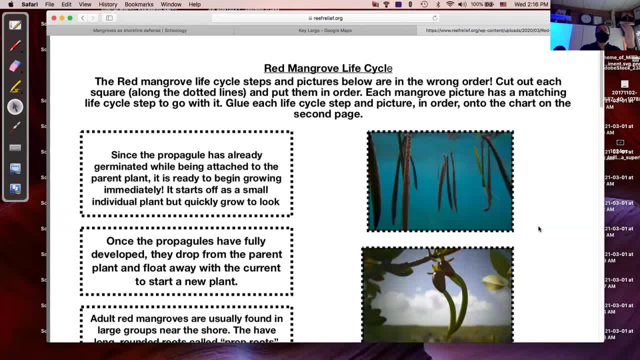 ever been to the central florida, southern florida, it rains regularly like it's like a. if you go to disney world, it rains like at least every other day, if not every day. so as the plant grows and gets salt on its outside surface, it just gets washed off by the rain, just as a natural. 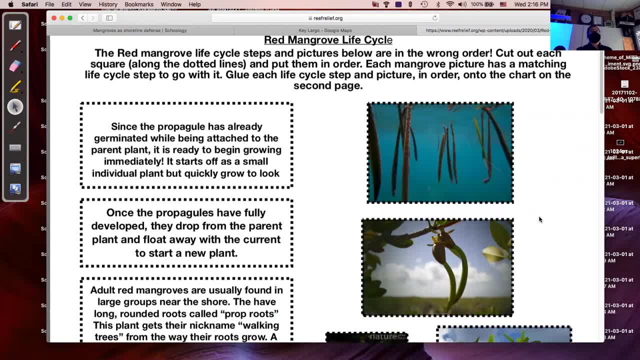 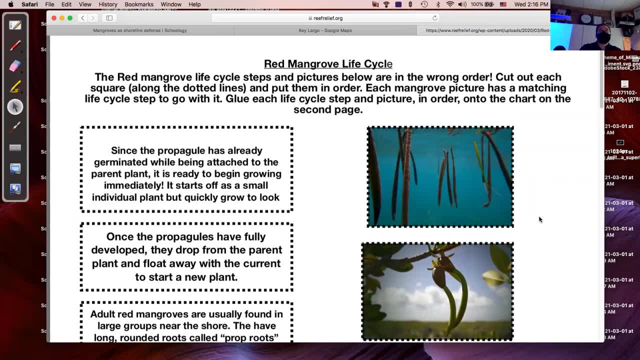 process. what i have to do back in that tank is there's i have a big water sprayer thing and i spray the plants down every day, and spraying the plants down not only sprays the salt off the plant but it also gives fresh water directly to the leaves. so it's less energy. it's difficult, it takes. 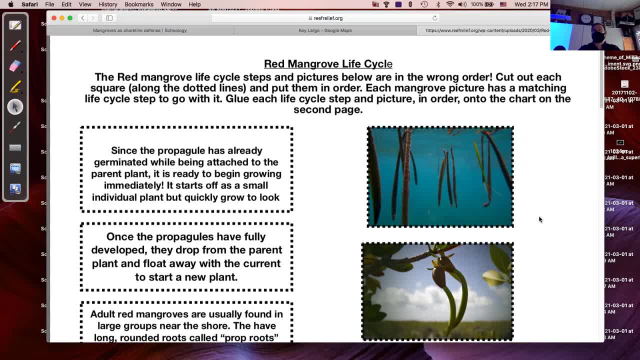 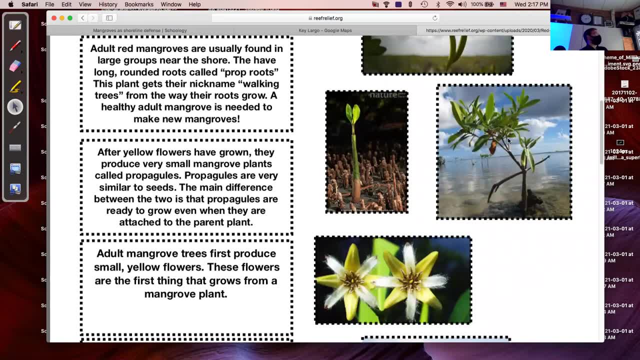 a lot of water out of the plant to take and separate water from salt from the water body itself. it's far more, uh, it's far healthier, for the plants. also spray water directly on the leaves. so i'm always spraying salt off the leaves and off the base of the tree in order to get them to grow. 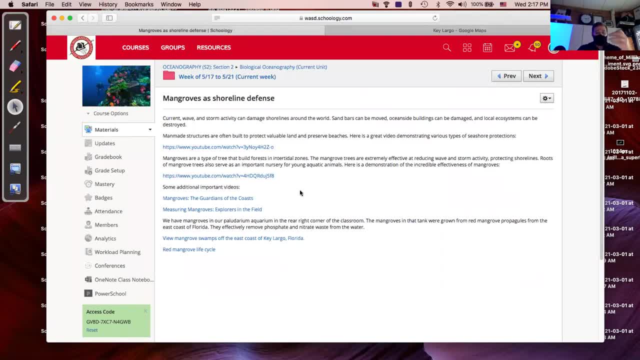 so, uh, mangroves are critical and just like in a coral reef, how they're like the rainforest of the of the steep of the seas and they're home for baby fish. they're very important homes for baby fish. baby fish can live in around there and provide some 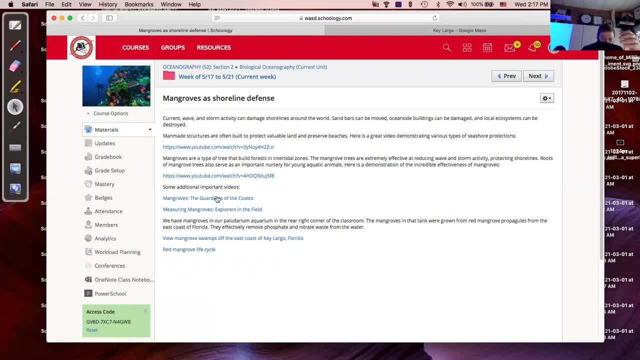 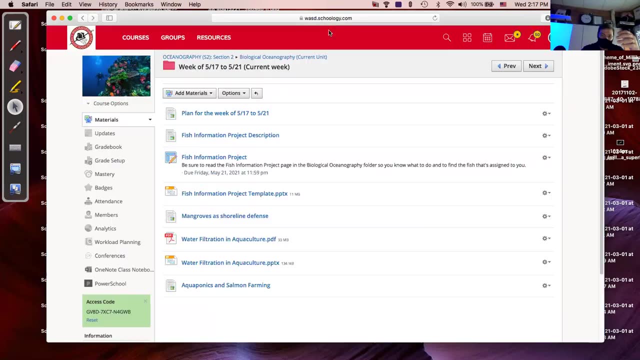 uh, protection, they're very, very diverse places. uh, i think that was it. mangroves- yeah, that was cool, i don't know. we're almost done. 2, 17.. tomorrow's a regular schedule. we go one to seven. let's see. the next week is monday, tuesday, right. 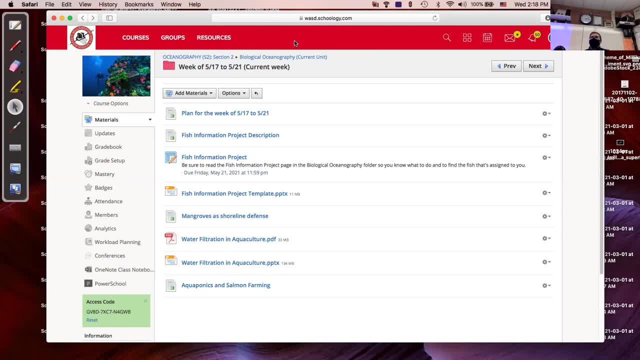 for the keystone bio. now we repeat the crazy schedule like one, three, four, two, five, six, seven, then one, six, seven, two, five, three, four. on monday and tuesday we'll do all of them. uh, if you didn't finish the fish information project, it's all working now. 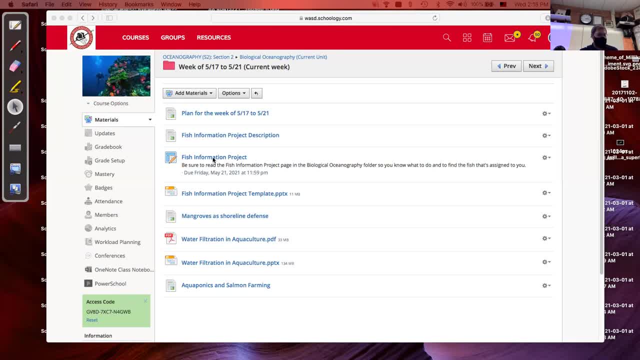 like i don't know why things weren't working. it was just a glitch with schoology and office, but they got it all fixed. so now the document will open and you can work on what whatnot. okay, Thank you. Is Malik skipping today? Is he taking a test or something? He didn't come. He didn't come.